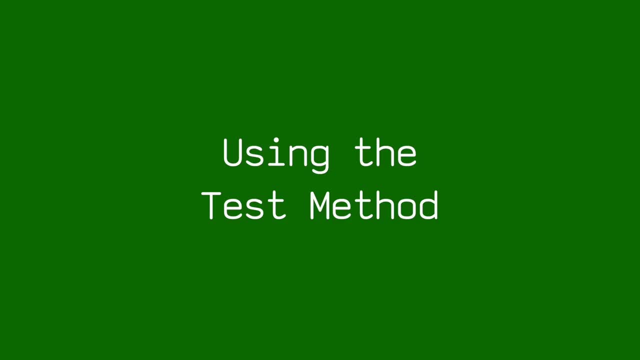 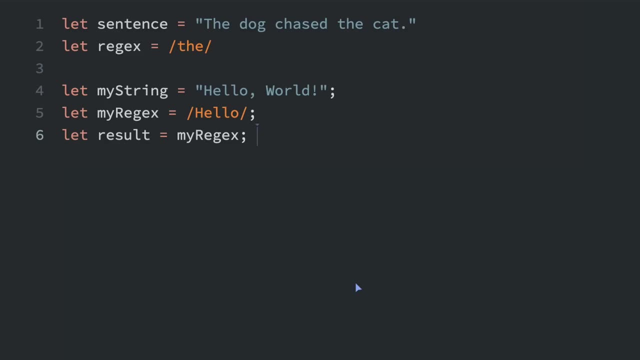 that's at. Well, let's get started. Regular expressions are used in programming languages to match parts of strings. you create patterns to help you do that matching. So, for instance, if you have the sentence the dog chased the cat and you want to match the word the, you can use this regex. here you can see that there's a slash and the word the and another slash. you will also notice that quote. 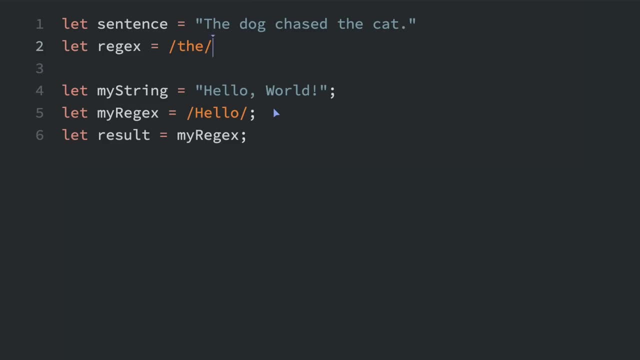 mark are not required within the regular expression. So JavaScript has multiple ways to use regexes. One way to test the rejects is to use the test method. The test method takes the rejects, applies it to a string and then returns true or false if the pattern matches something. So in this example we have the string Hello world, we have this rejects And we have my rejects. I'm going to do dot test And then, inside the parentheses, 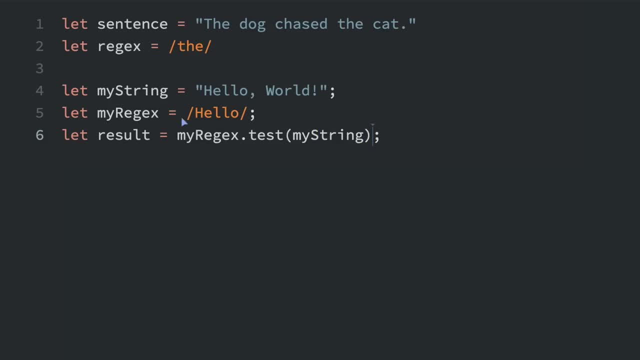 I'm going to put my string. So we are going to see if my string contains this: rejects, which is Hello, and then we'll put it into the result. In this case, it will be true, because Hello world does contain the string Hello. 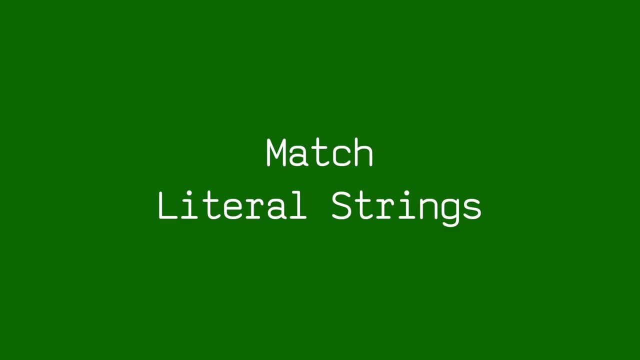 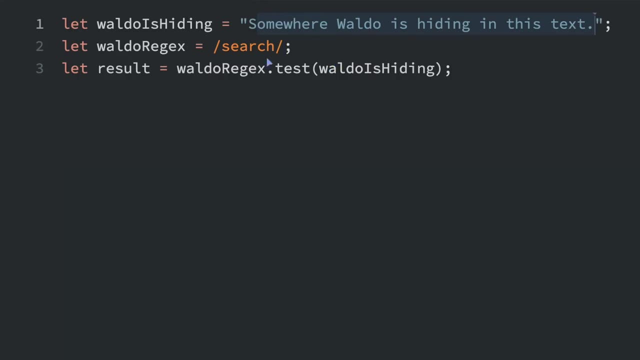 So here we want to match the word Waldo. we have this sentence somewhere. Waldo is hiding in this text, So I'm going to change this: rejects instead of search. it's going to be Waldo. Now. one thing I want to point out is that this is case sensitive. So if I had a lowercase w, 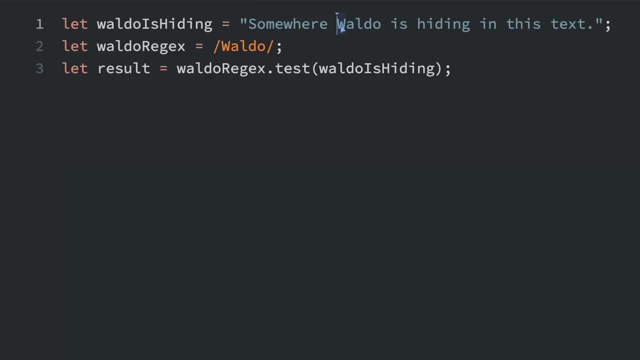 then this would not match. But since this starts with an uppercase W, I have to make the regex start with an uppercase W also. So this result- the Waldo regex dot test while Waldo is hiding- is going to return. true, because it found Waldo in this sentence. 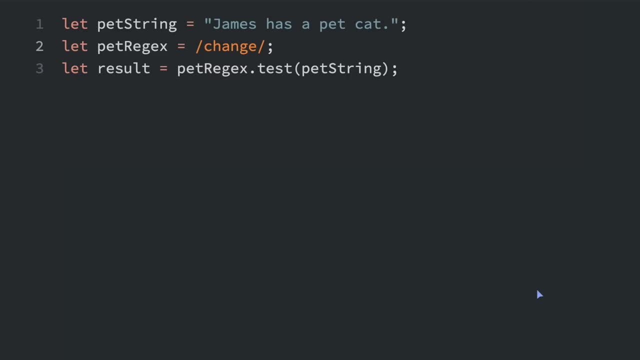 regex has an or operator which is a single pipe character. So in this example, let's say we want to try to match for multiple words Instead of just a single word. let's say we want to match dog, cat, bird or fish. So what I would do here is I'm going to change this, I'll do dog and then 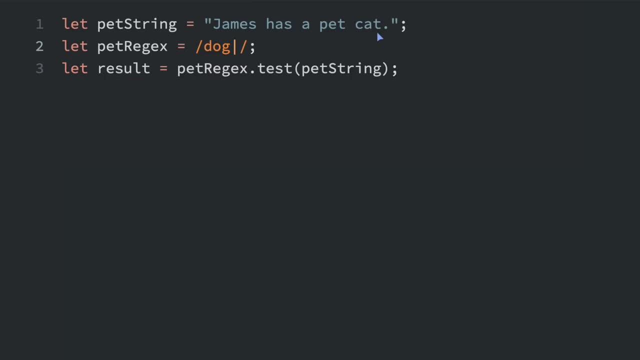 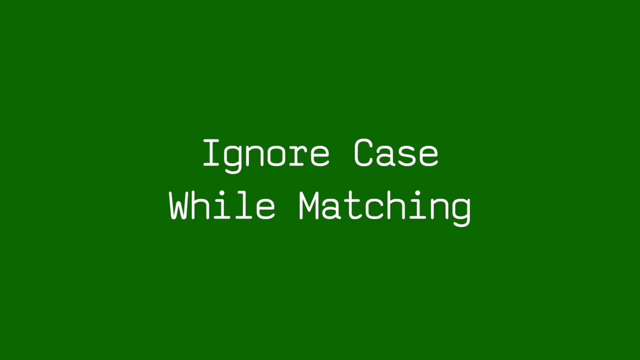 I'll put pipe which is just a straight line up and down, And then I'll do cat pipe, bird I fish. So this is going to match any of these four words: dog or cat or bird or fish. And since one of these words is in the sentence, this test is going to return true. So far, all the regexes. 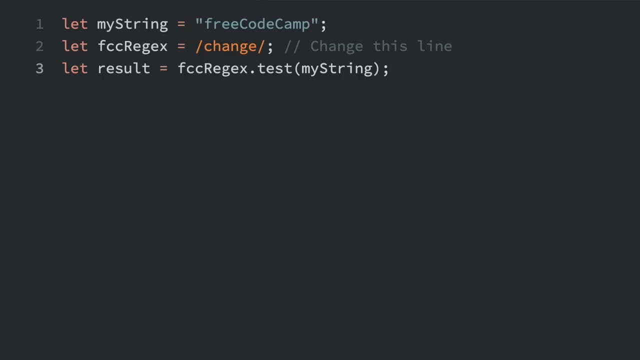 we looked at matched literal strings, So the case mattered If it was a capital letter. that's completely different From a lowercase letter. you can match both cases using what is called a flag. So there's the I flag that ignores case. So let me show you how you would do that. Let's say we have free code camp. 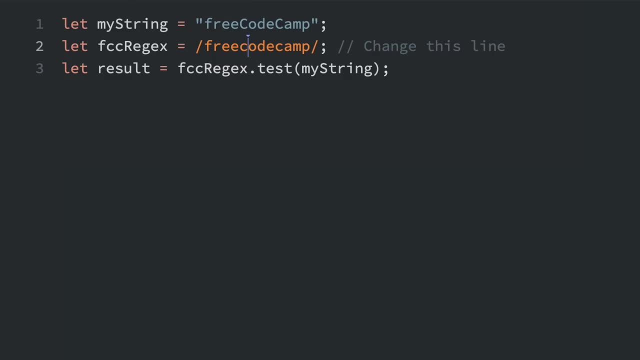 And we'll see. it's all lowercase in here, but we want to match it, no matter what the case. So we want this to also match this, where there's a capital C and another capital C. So just after the last slash I'm just going to put an eye. So this is the flag. This means ignore case. So now, when it, 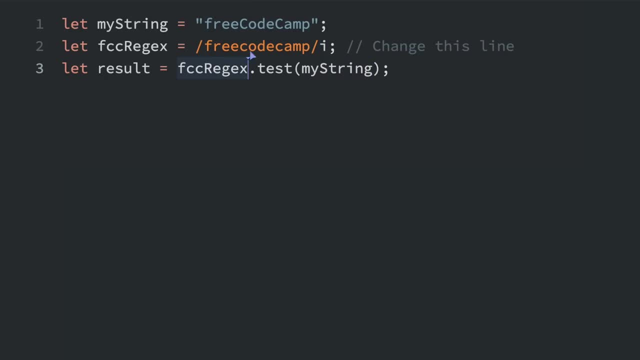 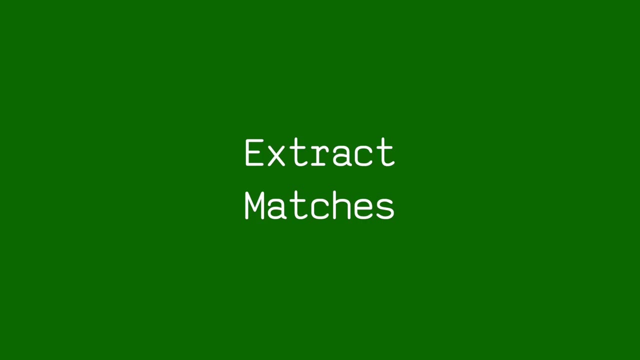 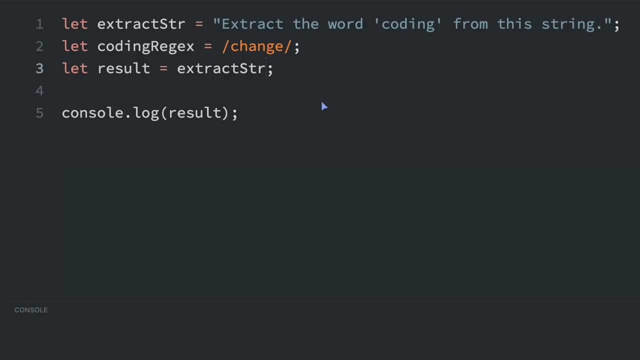 tests the string free code camp for the rejects, which is free code camp all lowercase. the result will be yes, because they will match So far. we have just checked if a pattern exists or not within a string, But we can also extract the actual matches that we found with the match method. 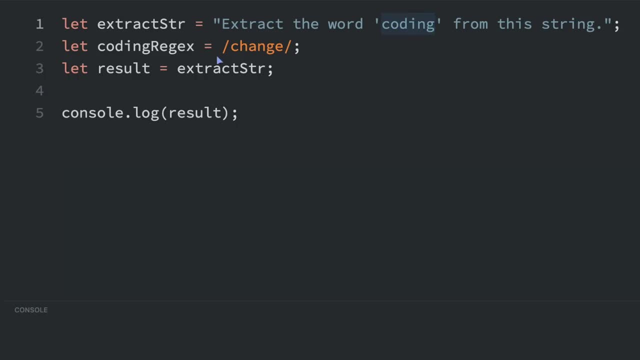 So let's see how to extract the word coding from the string. So we'll just change this to coding And then here we'll use the dot match method match, And then in the parentheses we'll pass in coding rejects And then if we just run this, we'll see in the console coding, because it's. 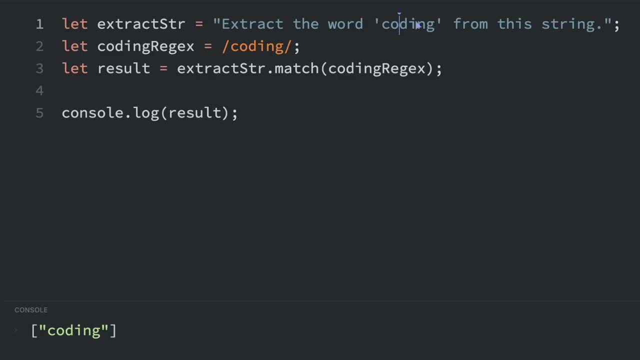 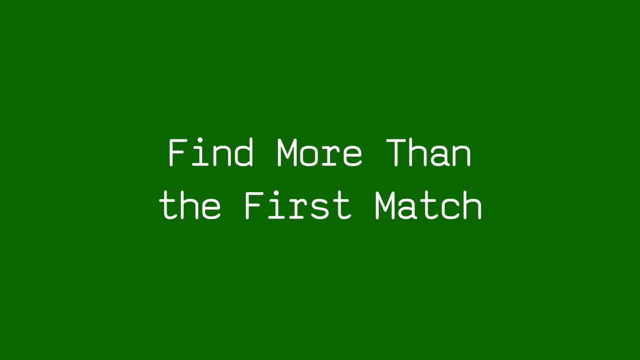 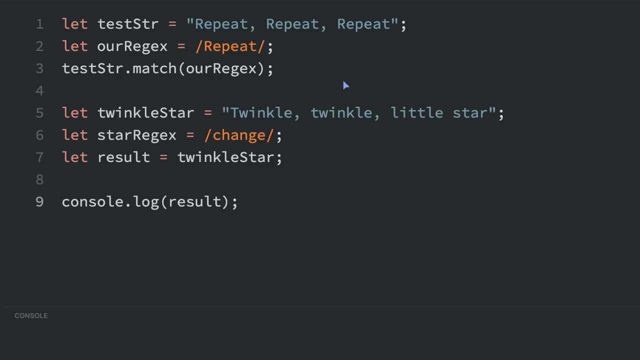 logging out the results. see the result extract of this. we're coding out of the sentence and into the result variable and it got logged. So far we've only extracted search patterns one time, But it is also possible to search or extract a pattern more than once using the G flag. Let me 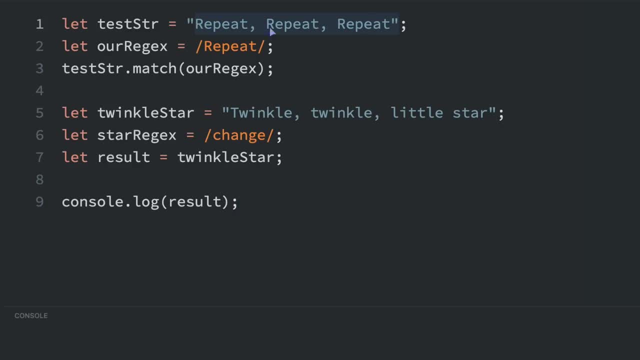 show you what I mean. We have this test string up here: repeat, repeat, repeat. Now we're going to just search for repeat And the way it is now, when it matches this, it's only going to return the first repeat, just this one. But if we add the G flag after the slash here, it's going to find every. 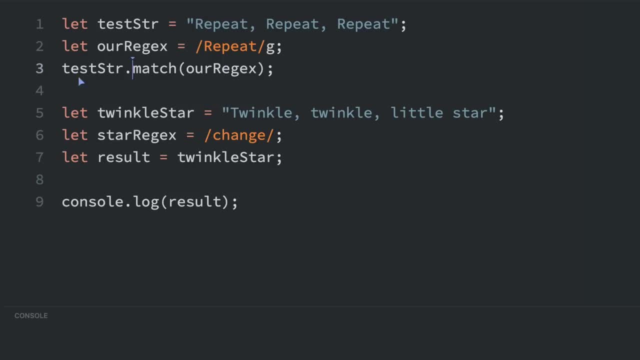 single occurrence of the word repeat. So it's going to return an array with three elements And each element is going to be the word repeat. Let's see it again down here where it says twinkle, twinkle little star. I want to match. 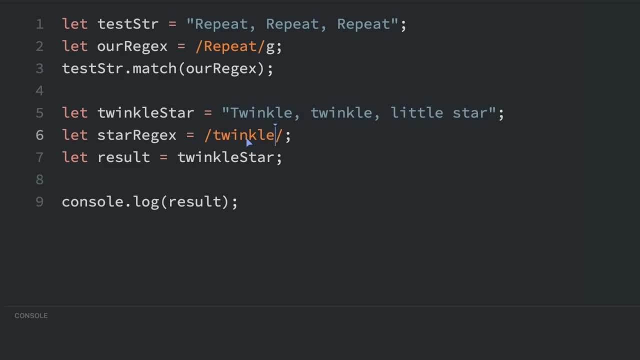 the word twinkle. So I'll type in twinkle right here And you'll see that the first twinkle is capitalized. the second one is not. So I'm going to have to use a flag. I'll have to use the I flag. 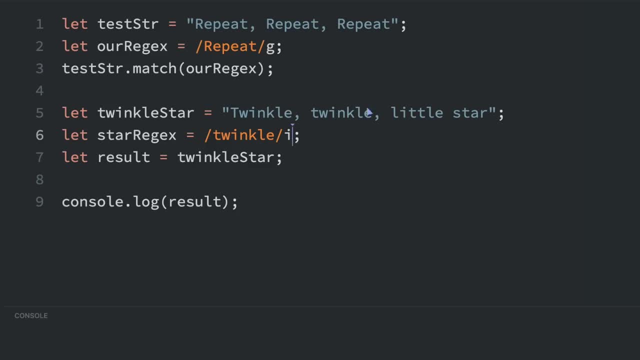 which makes it insensitive to case. So it's case insensitive. I'm also going to add the G flag that's going to match every single time twinkle appears, So you can use two flags at once on the same regex. Now here for the result. it's going to say repeat And it's going to return an array. 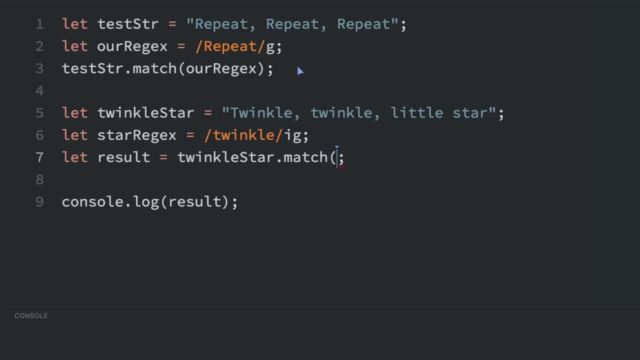 that's going to be twinkle star dot match And then I'm going to pass in the star regex. Okay, now we'll log this and see what happens. You can see twinkle, twinkle. the first twinkle in the console is the capital T and the second is the lowercase, because it matched the first one. 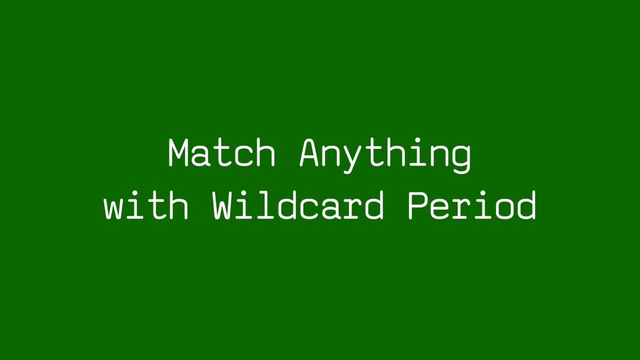 and the second one and return them both In regex. a period is a wildcard case, So it's a wildcard case. In regex, a period is a wildcard case, So it's a wildcard case, So it's a wildcard case So. 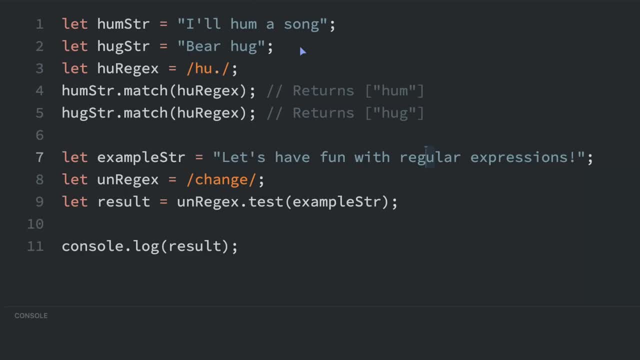 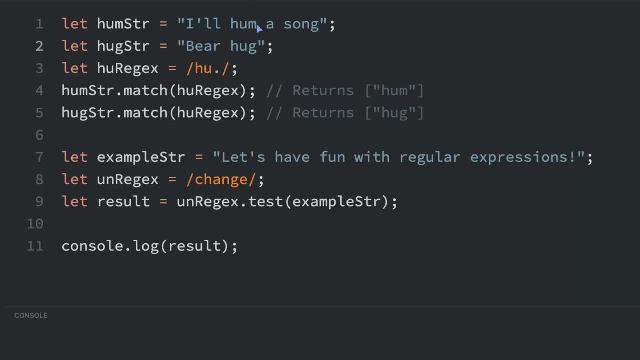 start with the same two letters, hu, And then the third letter is different. So look at this regex here: hu, period. this will match any word that starts with the characters hu and then then has a final character, which could be any character, And then the third letter is different, And then 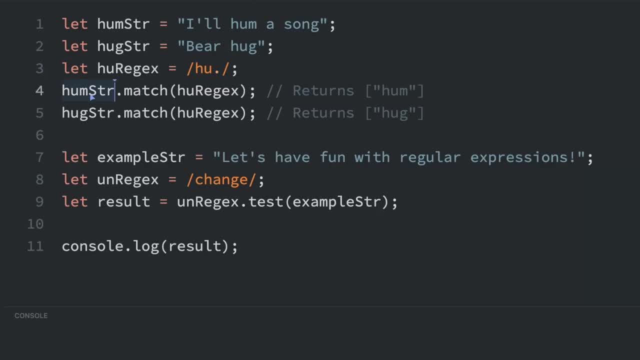 then has a final character, which could be any character. So if we look down here, we are going to take the first string- I'll hum a song and match it to our regex. it's going to return hum. And then when we take our second string- bear hug- and match it to our regex, it's going to return. 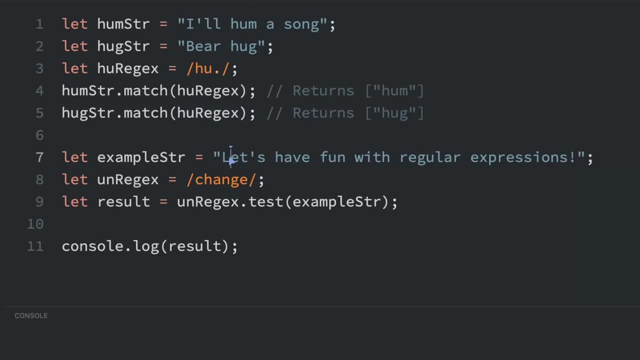 hug. So let's try that with another sentence. We have this sentence here, Let's have some fun with regular expressions. So I want to match the word fun. But I also want this regex to be a fun word. regex to be able to match the word run, son, pun, none or bun, basically any word that ends with. 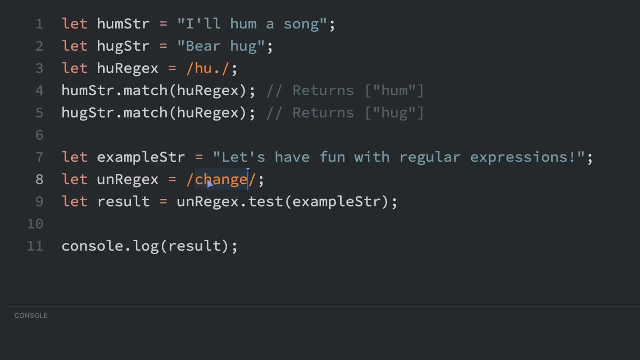 you in and starts with another letter. So I'll change this regex to dot u n. So when we run our regex and search this sentence for something that ends with you in, it should find fun. So let's load that and look in the console And it says true, because it matched the word fun. 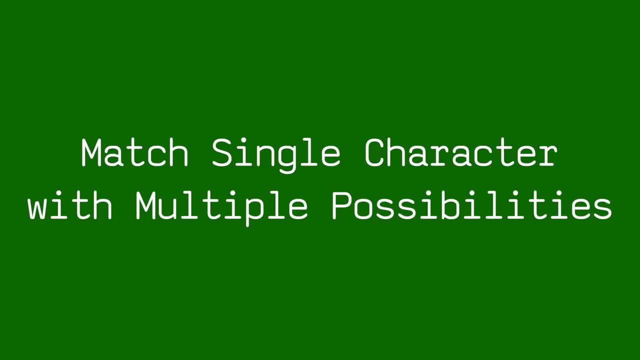 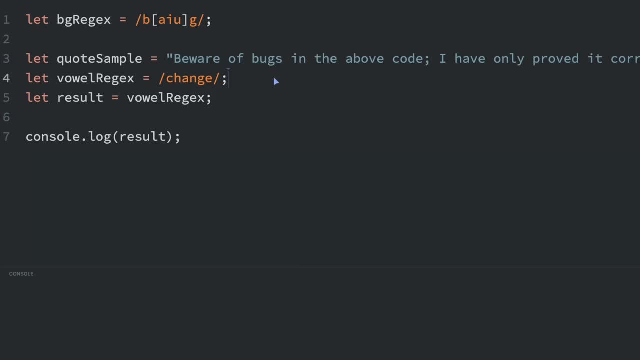 that sentence We talked about the wildcard character, which matches basically anything, But you can also match from a predefined group of characters. If we look at this right here it we have the B and then we have these brackets, And inside the brackets we're saying that the second letter, that 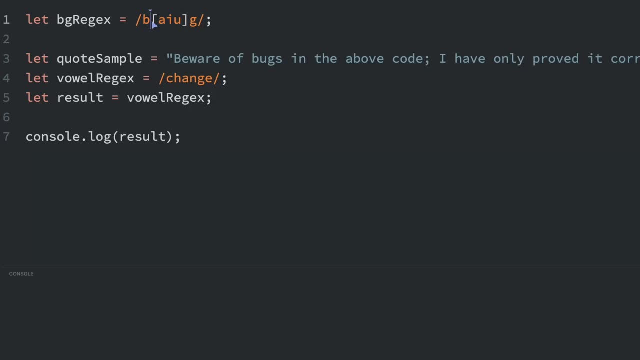 is going to match has to be one of these three letters. So we know the first letters going to be B 00.. last letter letter is going to be G and the middle letter is going to be a, i or u. So this would match bag big. 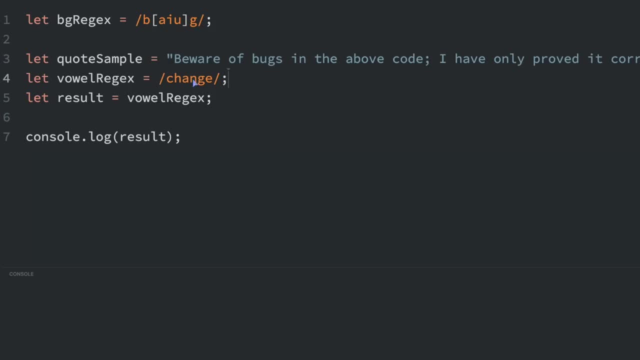 and bug. So down here, what we want to do is change this So we match every single vowel in this quote sample here. So what I'm going to do is put open and close brackets And inside I'm going to put the vowels A, E, I, O, U And then to make sure I match every single vowel and I match uppercase. 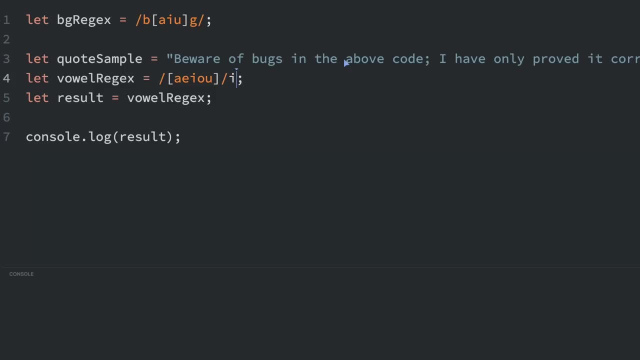 or lowercase vowels. I'm going to use flags. I'll use the I flag and the G flag. Now down here I'm going to have to do quote sample dot match And then I just pass in the vowel rejects. here I run. 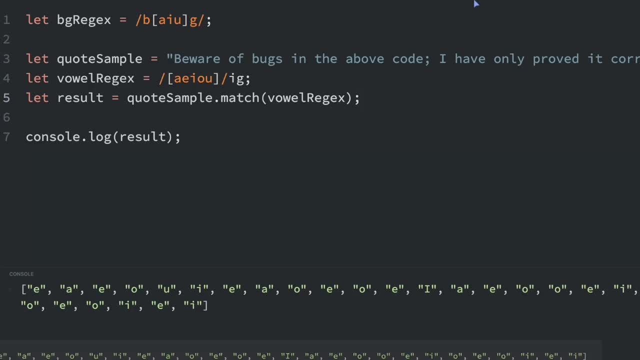 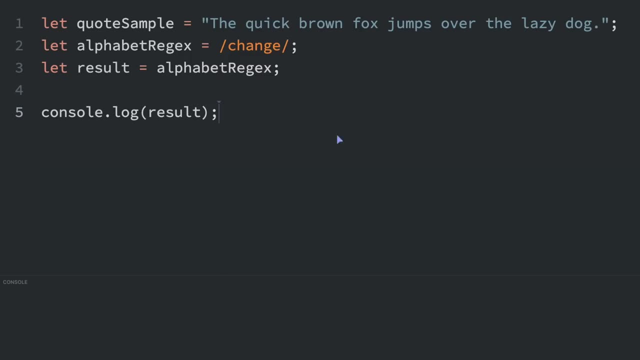 this: in the console you'll see all the vowels from that quote sample. You can also match a range of letters. So I'm going to go ahead and do that, And I'm going to go ahead and do that, And I'm going to go ahead and do that, And I'm going to go ahead and do that. So let me show you how to do. 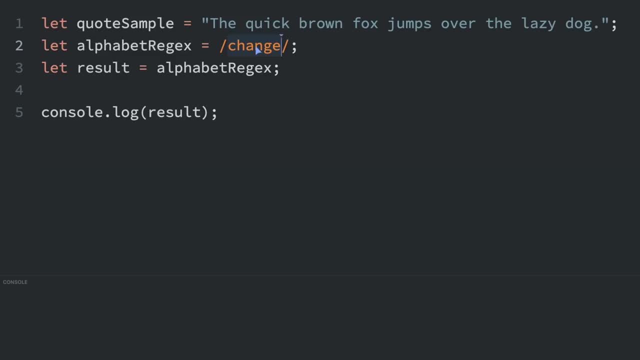 that Right here I'm going to try to match every single letter. So I'm going to put the open and close brackets And instead of typing ABCDEFG and writing every letter, I can just put A through Z, So it's going to match every letter between A and Z And then to make sure it matches every. 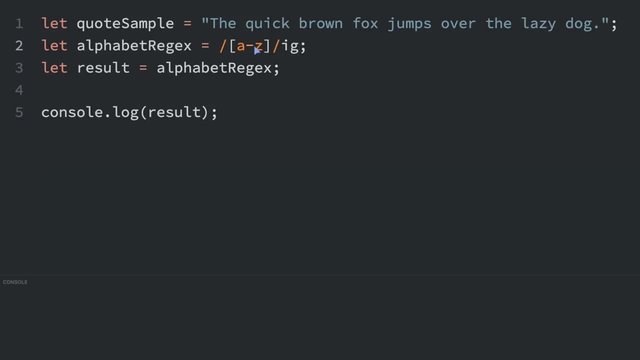 uppercase and lowercase letter, I'll do I and then G to make sure it matches every letter in the whole string. So now I can just do that And then I'm going to go ahead and do that And I'm going to do quote sample match And then I just pass in the alphabet regex here. And if I run that, 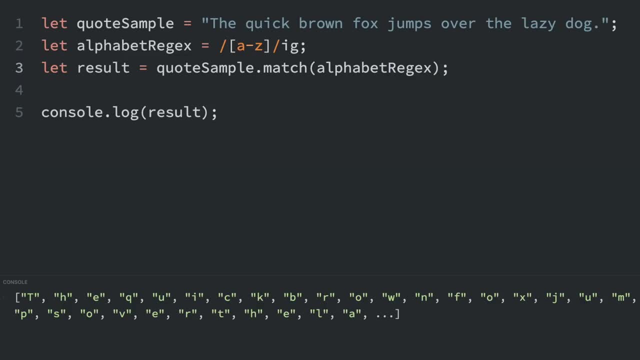 we would see in the console, it has every letter in that string. Just like you can use a regex to match a range of letters, you can also match a range of numbers. So if I want to match range of numbers, it will be like this: I'll have the brackets here, the opening and closing brackets. 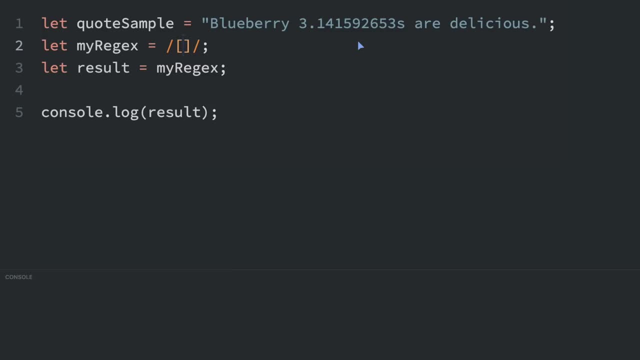 and this time I'm just going to match the numbers two through six. So I'll just put two dash six, So that will match 23456.. Also in the same regex I can match a range of numbers and a range of. 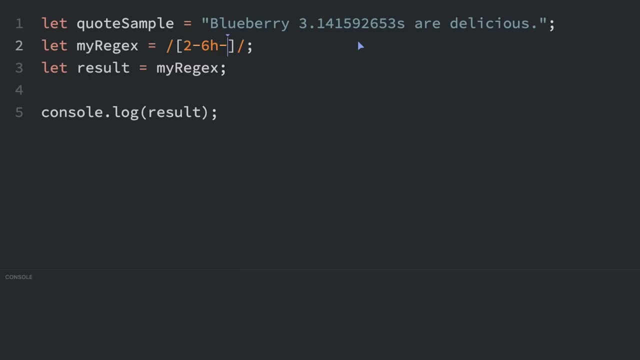 letters. So if I want to add some letters I can put h through s. So now we can see this is going to match a range of numbers two through six and also a range of letters h through s. So I can do an eye to make it case insensitive And then I'm going to go ahead and do the same thing here. So 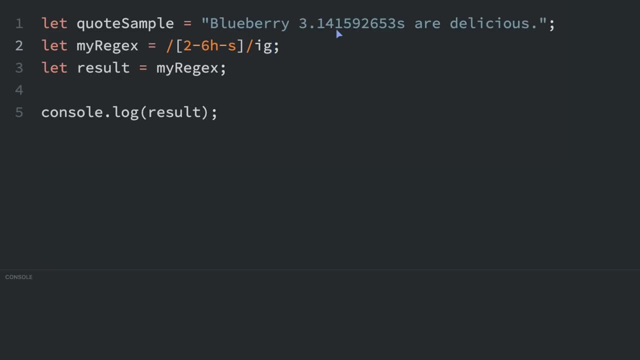 I'm going to go ahead and add a g to match every occurrence in the whole string. So I'm going to put that into my results. So I'll do quote sample dot match to match this regex And here it's going to console dot log the result. So let's see what happens And we have every letter. 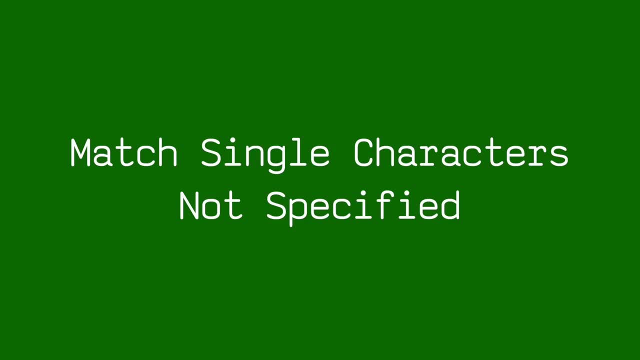 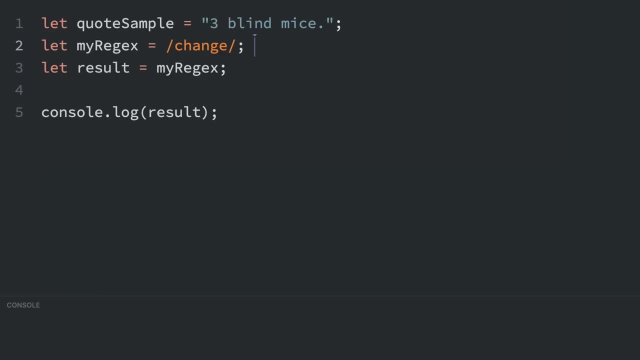 and number between those ranges. We've talked about how to match for specific characters, But what if you want to create a set of characters that you do not want to match? These are called negated character sets, And you can create them with the carrot character. So let me 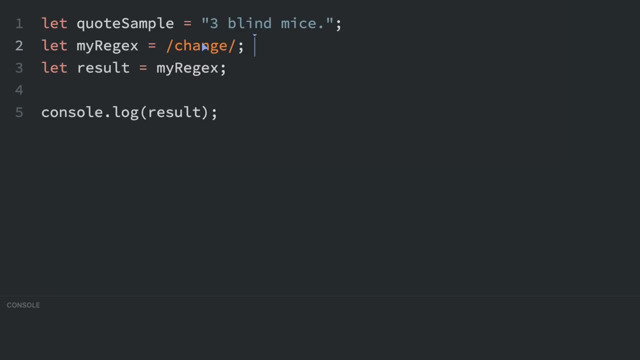 show you how to do that This. we want to make a regex that will match everything except all numbers and all vowels. So we are going to put a open and close bracket And I'm going to put a carrot character And I'm going to put a character character And I'm going to put a character character. 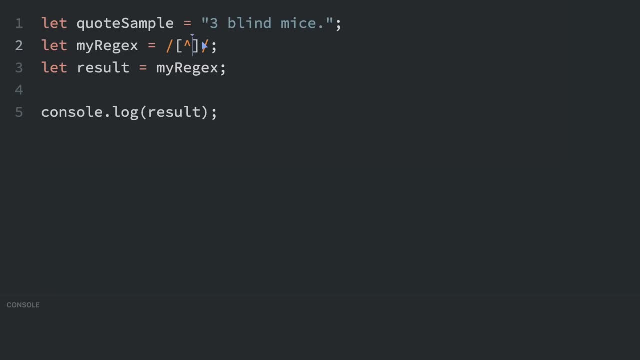 that's right underneath a six on a keyboard, And I'll put zero through nine. So we are not going to match all digits zero through nine, And we are not going to match a, e, i, o, u, And then I will put my flags here. i, g, So this will match everything except zero through nine and a, e, i, o, u, So to 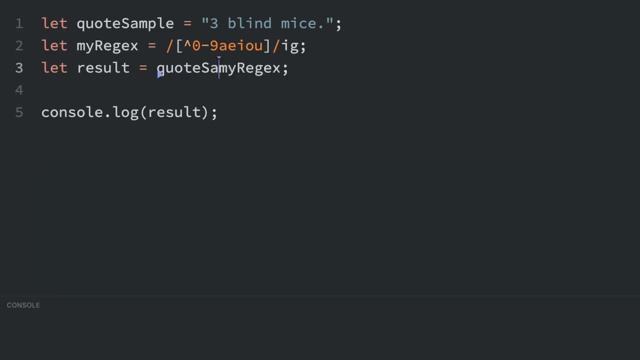 finish this up, I'm going to put quote: sample: dot match And then I'll pass in the regex here And now I'm going to go ahead and add a regex here And I'm going to put a quote: sample: dot match. And. 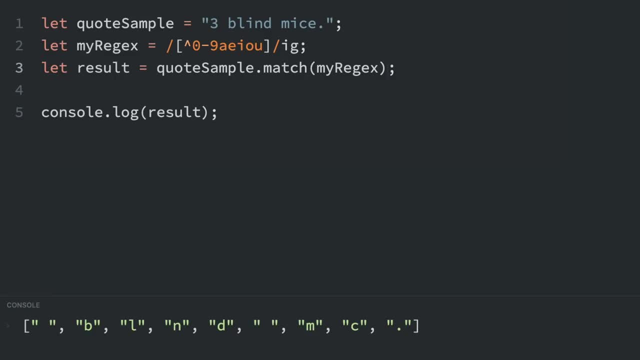 now I'll just run this And you can see we've returned everything except the vowels and numbers. It includes the spaces and periods and punctuation also. Sometimes you want to match if a character occurs one or more times. If you want to do that, you can use the plus character. So let me show you. 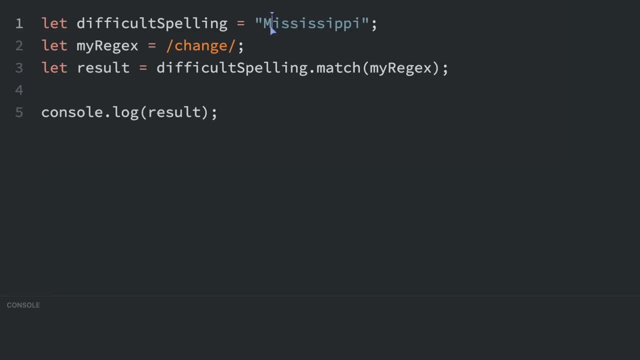 how to do that In this case. we are going to try to match in the word Mississippi whenever an s occurs one or more times. So I'm just going to put s plus and I'm going to put a G to match it. 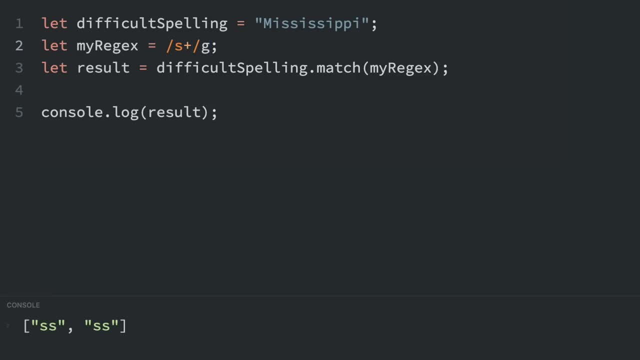 every time it occurs, And if I run this, you'll see we've matched the first SS and then the second SS. If there just happened to be another s in here, we would then match three times And you can see. the third time only matches the single s, because there's only one s in a row, And 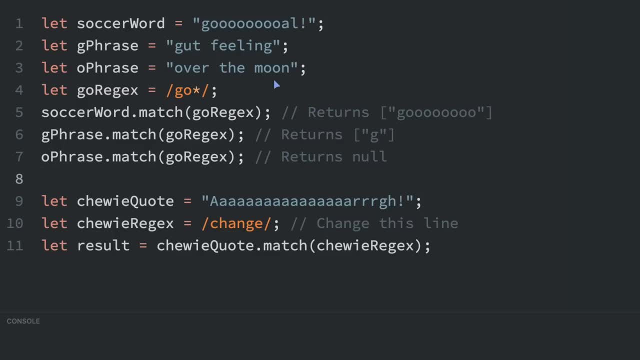 there is an option to match characters that occur zero or more times. That's with this star character here. So this rejects means match a G and then match an O, zero or more times. So with this word goal it's going to return G, O and then every O after it, And then here, gut feeling. 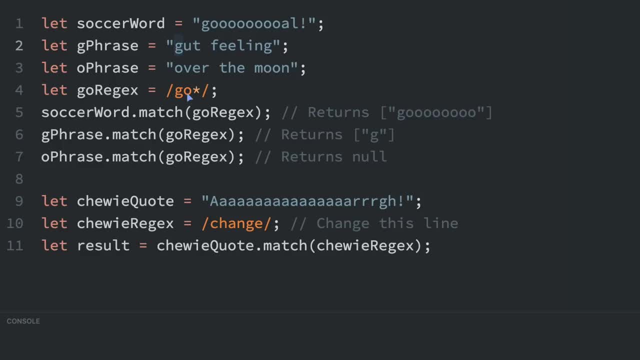 there's a G with no O's after it And since it's matching zero or more times, it's going to match that and just return G. Now, this one has no, it has an O's but it doesn't have a G, So it's gonna return. no, it's not going to match at all. So down here we are going to do. 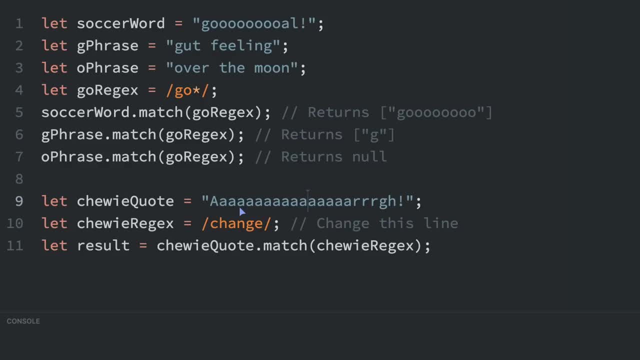 some coding and match a zero or one time. So I'm going to change the change word here And we always want to get the capital A and then for the lowercase a we are going to do a asterisk So it can match it. 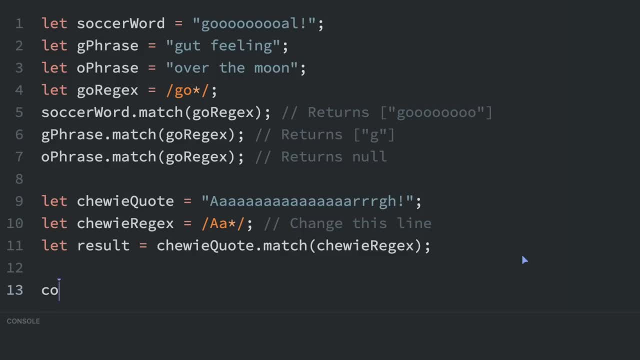 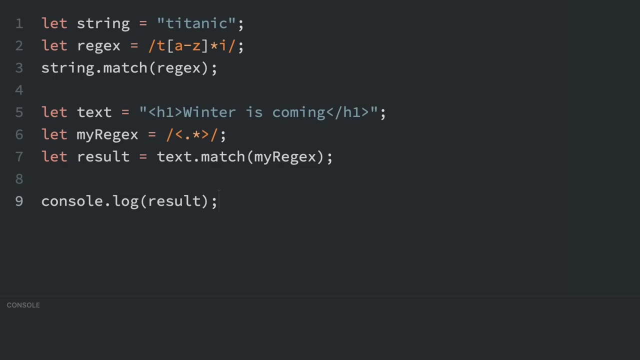 This whole thing of A's here. So if I just do a console dot log here and do a result, it should match all of the A's. It worked. I am going to talk to you about greedy and lazy matches. A greedy match finds the longest possible. 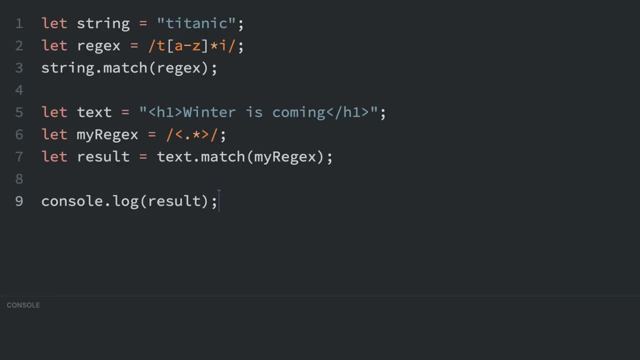 part of the string that fits the regex pattern and returns it as a match. A lazy match finds the smallest possible part of the string and returns that regex patterns default to greedy. Let me show you what I mean. Let's look at the string here- Titanic- And we'll look at this regex to find. 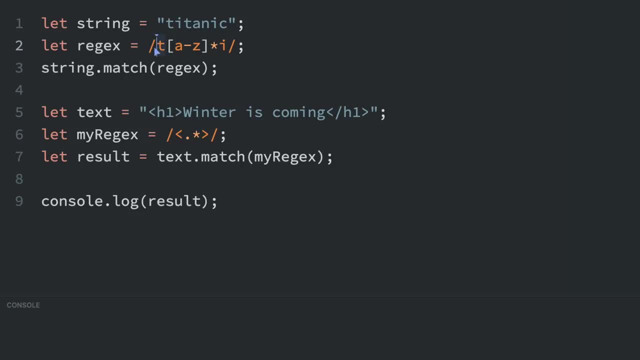 something in the string Titanic. First we're looking for the letter T And then this part means, after the letter T, we want zero or more of any letter. So remember this means any letter A through Z. the asterisk or star means zero or more occurrences of this A through Z, And then 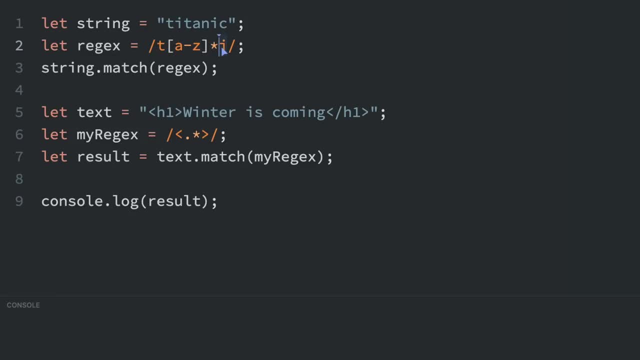 finally, we're looking for a letter I at the end. So when we run this match here, it's going to do a greedy match and find this ti t a n i. So it's going to start with a T. it's going to have zero. 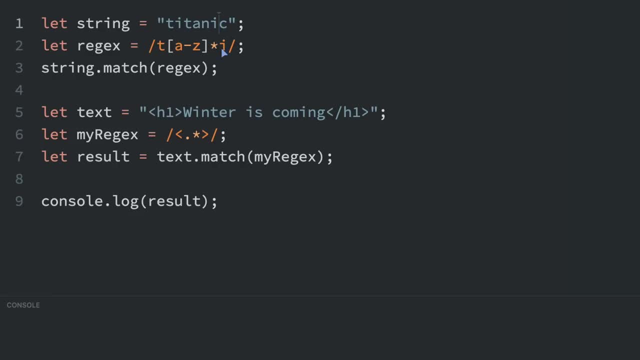 or more letters and in with an eye. However, if we put a question mark here, it's going to be a lazy match. So it's going to start with the T And then remember this is zero or more occurrences. So instead of having all these letters, we're going to go to the zero occurrence. 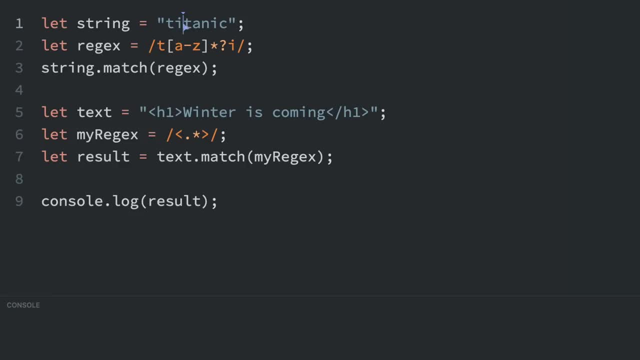 and not have any letters and then end with this: I here, So it's just going to be ti. So a greedy match would be ti t a n i. a lazy match would just be ti. So let's do the same thing down here We're. 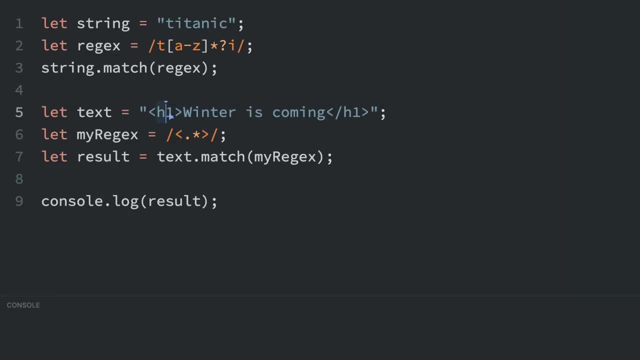 going to run this match And then if we start with a string here which is a bit of HTML, with an h1 tag, some text- winter's coming and a closing h1 tag, If I run this now, you'll see in the console. 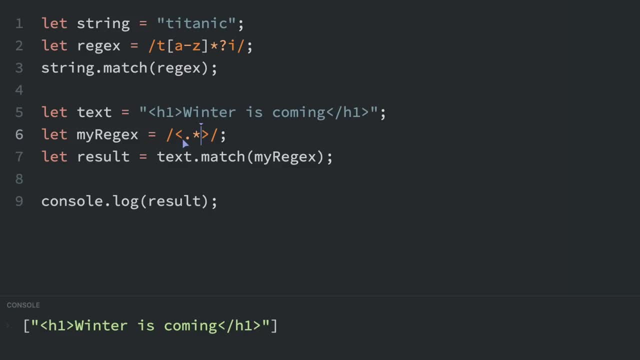 it's going to return the whole thing. So we're going to start with the more than sign here, And then we have the dot, which is a wildcard character, So this means any letter or character. and then the star or asterisk means zero or more occurrences, So this means zero or more occurrences. 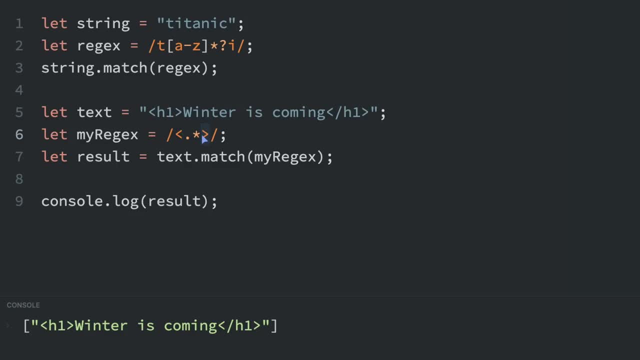 occurrences of anything, And then we end with the greater than sign. So we're going to start with the less than sign right here. this is to open an HTML tag And then we have the dot, which is a wildcard, the asterisk or star, which means zero or more occurrences. So when you have a dot, asterisk, 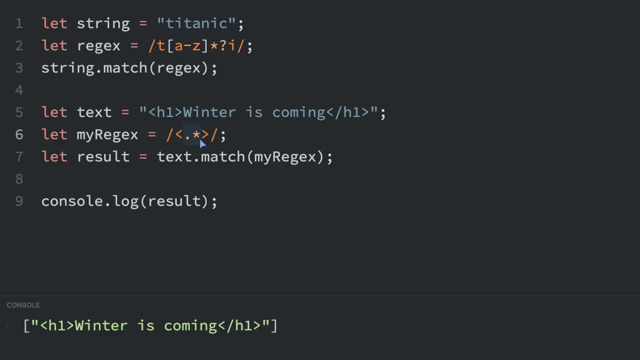 that means zero or more of occurrences of any character and then end with the more than sign or the closing tag here. So it's going to go from here And that's going to have zero or more occurrences of any character all the way to this final character here, this greater than sign. So 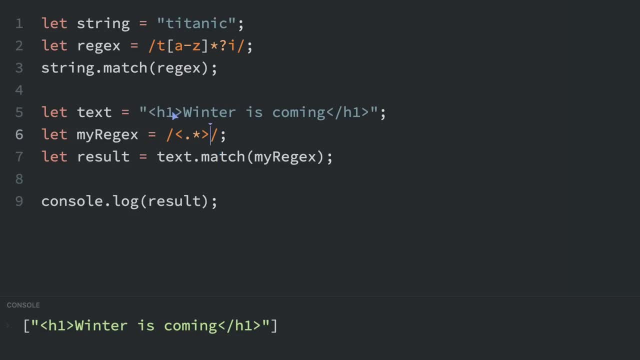 what we're going to do is change this. So, instead of instead of getting this whole thing, which was, which is greedy- we want to do a lazy match where it starts here and just ends at the first occurrence of this greater than sign. So all I have to do is change this to greater than sign. 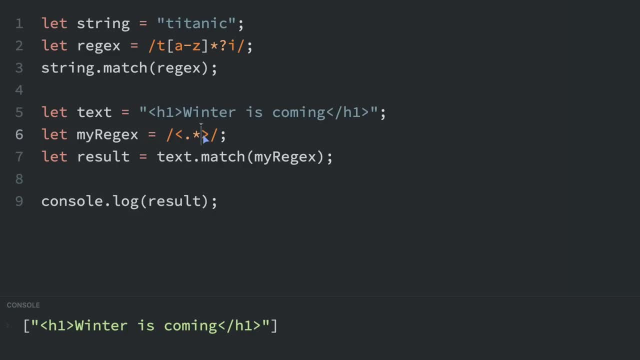 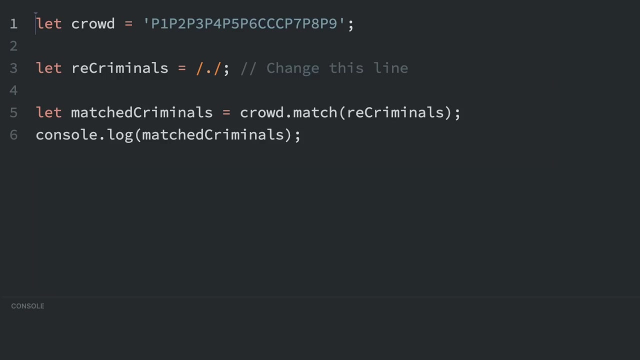 do for that is to add a question mark. So if I run this now, you'll see in the console it just has the opening h1 tag. This is a basic regex challenge. So here is the scenario: a group of criminals escaped from jail and ran away, but you don't know how many. However, 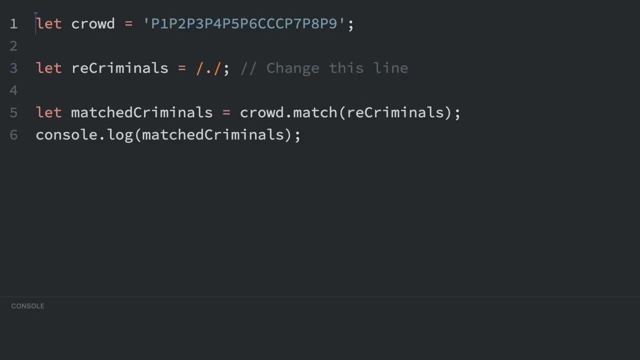 you do know that they stay close together when they are around other people. you are responsible, And that's what we're going to do, And then we're going to add a question mark. So that's what we're going to do, And then we're going to add a question mark. So, if I run this now, 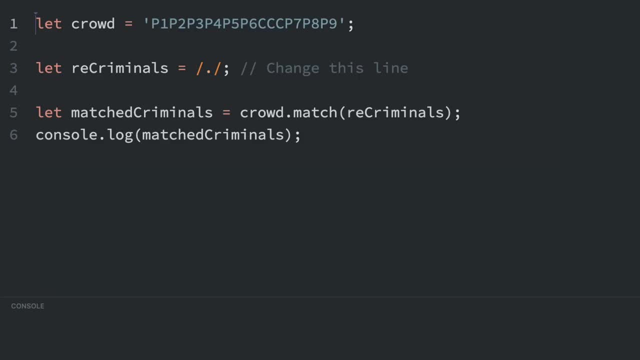 you're responsible for finding all the criminals at once. So the criminals are represented by a C. So you can see, here we have these three C's together. these are all the criminals. So we need to write a regex function that's going to match any times there's there is one or more C's. 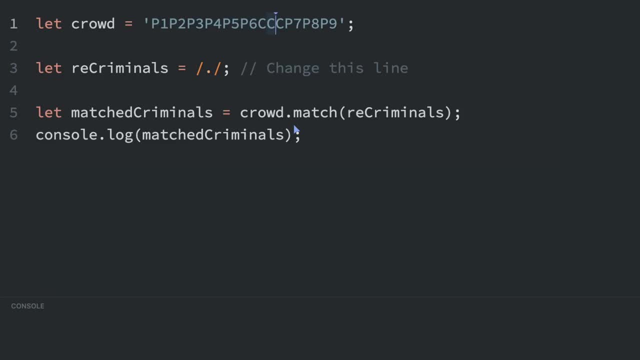 in the string that's passed in. So this is how you would do it. It's actually pretty simple. We're just going to run this And then we're going to add a question mark And then we're going to add a regex function that's going to match any times there's there's one or more C's in the string. that's. 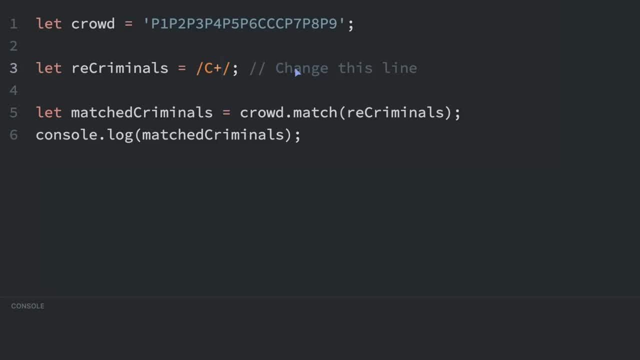 passed in. So this is how you would do it. And then we're going to add a regex function that's going to put a C and a plus, So it's going to match one or more C's And if we load that, you'll see that it. 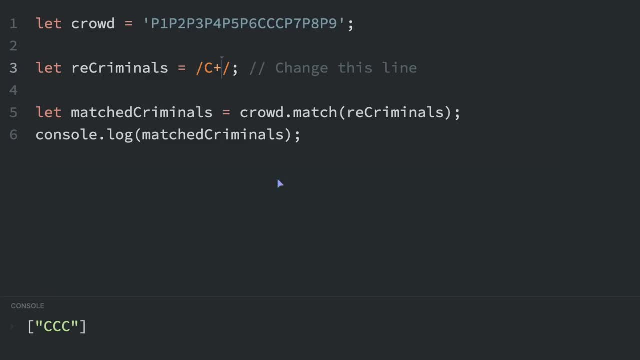 matches the CCC And we solve the challenge. You can match patterns that are only at the beginning of a string. Previously we talked about how the carrot character inside a character set is used to create a negated character set. Well, if you're not in a character set, if you're not in brackets- 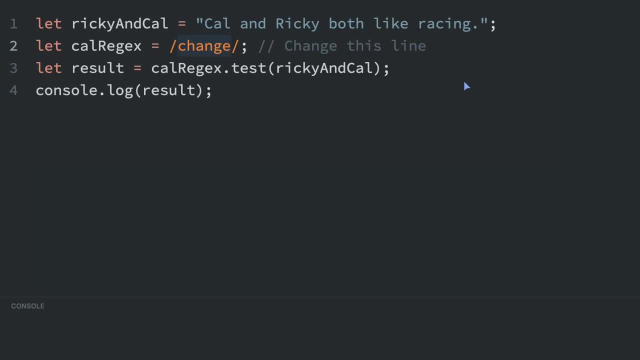 you can use the carrot character that looks like this to only match at the beginning of a string. So here I'm just going to match the word cow if it's at the beginning of a string. So if I load this you can see true, because it is the cows at the beginning of the string. However, 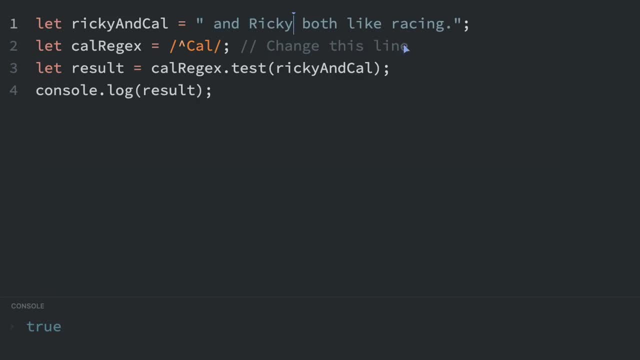 if I take the word cow off here and put it in the middle here And I reload that again, it's going to say false because it does not match it anymore, Since Cal is not at the beginning of the string. A carrot matches a. 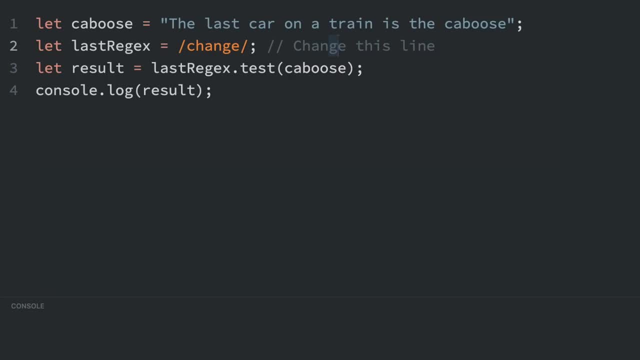 beginning string pattern. A dollar sign matches an ending string pattern. So if we want to match the word caboose at the end of the string here, we'll type in into the rejects, we'll type in caboose And then I'll put a dollar sign. If you remember when we were matching a beginning string pattern. 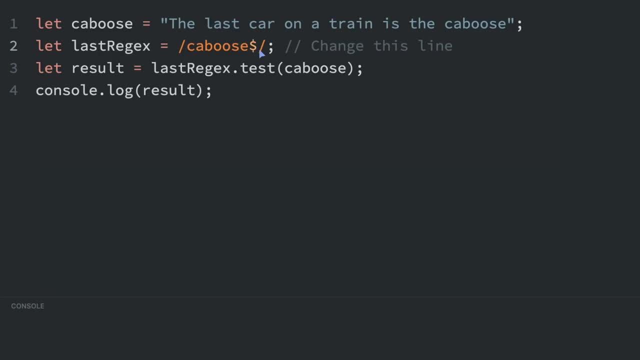 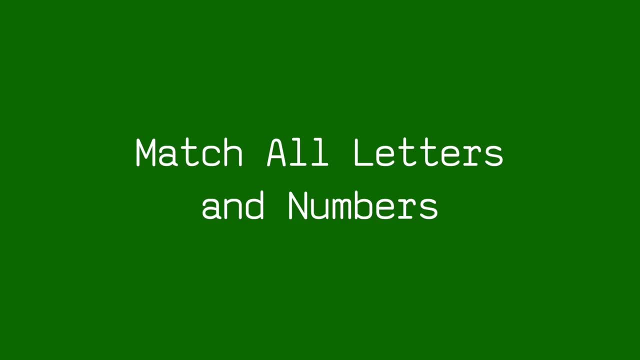 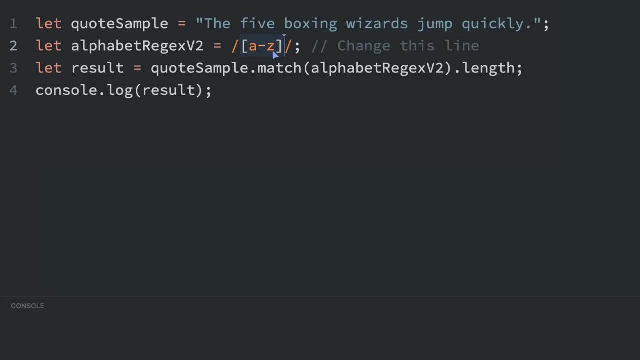 So it no longer matches caboose. Earlier I showed you that this, with the brackets and A through Z in it, would match any letter A through Z. There's something called a shorthand character class that's used to match a wide range of things And there's one called slash w that you can use to match the. 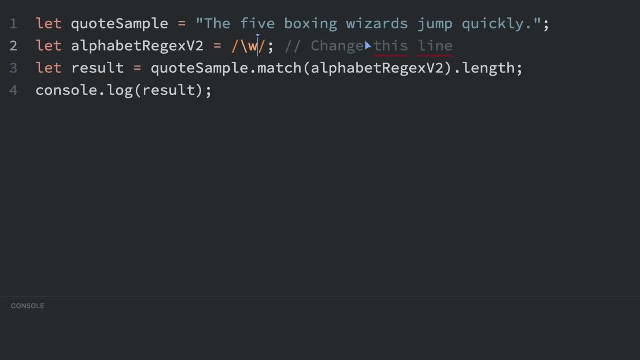 alphabet. So if I go to the alphabet I can match the alphabet And if I go to the alphabet I can. If I put slash w here, that's going to match capital A through z, lowercase a through z, the digits zero through nine and underscore. So just doing slash w is just a shorthand way of pretty. 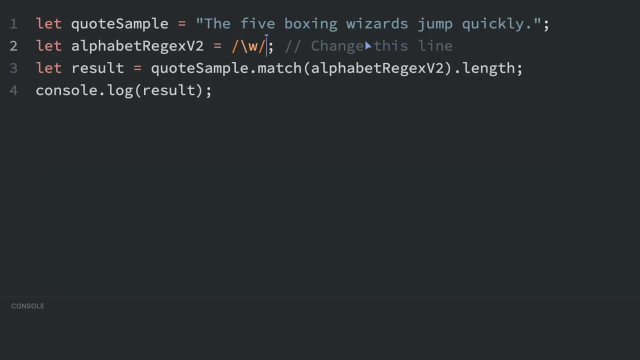 much matching any letter or number plus underscore. If I put a G after this, that will make it match every occurrence. So if I load this up, you'll see that it returns 31 because we're getting the length. the length of this whole string, excluding the spaces in the period, is 31.. There are 31. 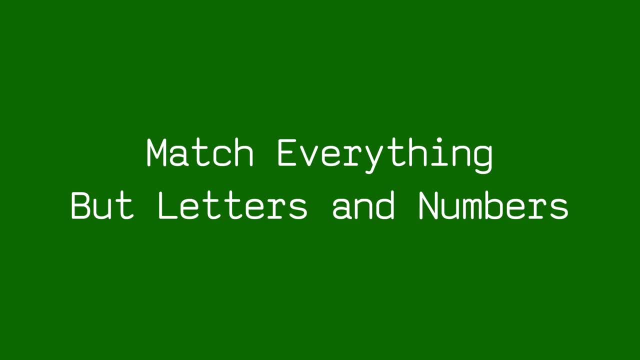 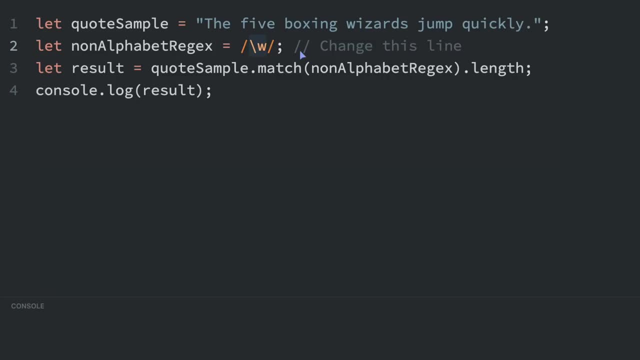 letters. in this string, Slash w matches all letters or numbers, But sometimes you want the opposite. Sometimes you want to match everything that's not a letter or number. So in this code we want to just match everything that's notал a letter or number, which are the spaces and the period in the string here. So instead 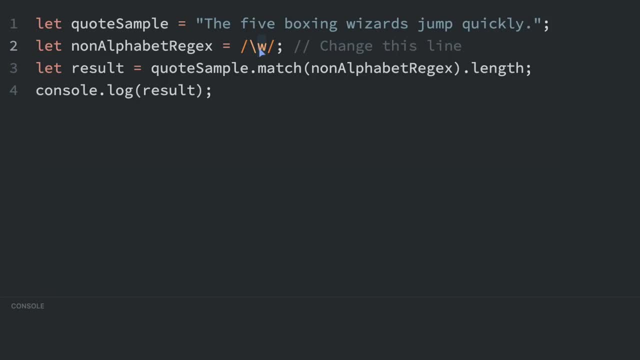 of a slash lowercase w, we're going to use a slash uppercase W And then I will put a G to match every single occurrence And we're going to get the length here. So if I run that we get a length of six. there are six characters. that those other spaces. 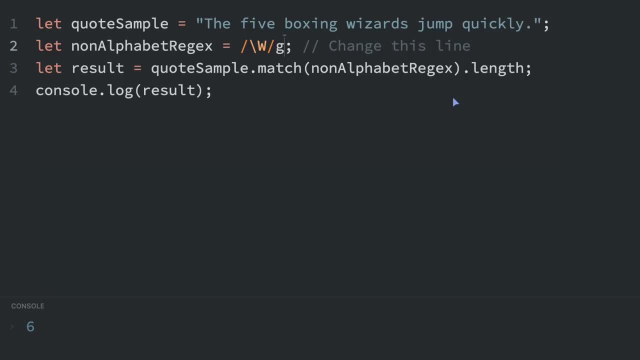 and the period that are not letters, numbers or underscores. There is a shorthand character class to only match numbers or digits And it's slash D. So if I put slash D here, it's going to match the digits here, which is the five, the zero. 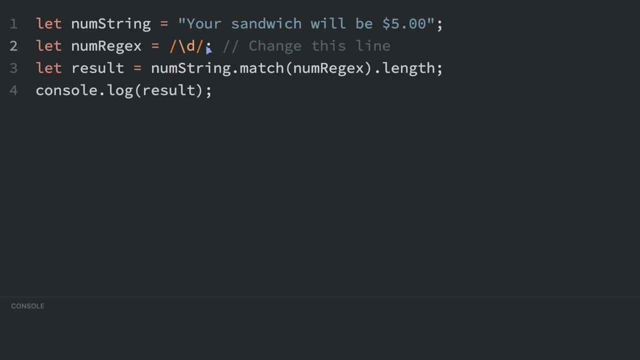 and the zero To match every single one. I'm going to put a G at the end for global And now the length should be three. So if I run that, we'll see three in the console. Sometimes you want to match all non numbers. If you remember this, slash d a lowercase. 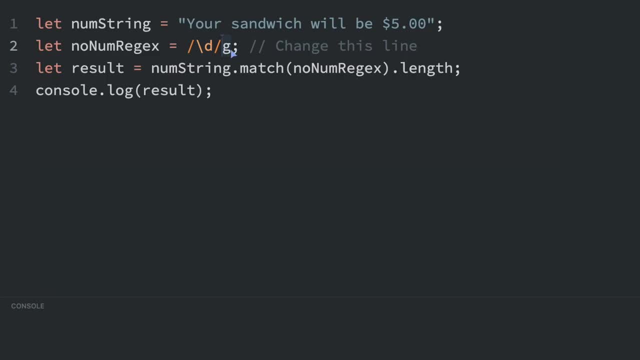 D would match all numbers and the G made it match every occurrence of a number. So if we change this to an uppercase D, this is going to match all non numbers. So that's going to be every single character in this whole string except the five, the zero and 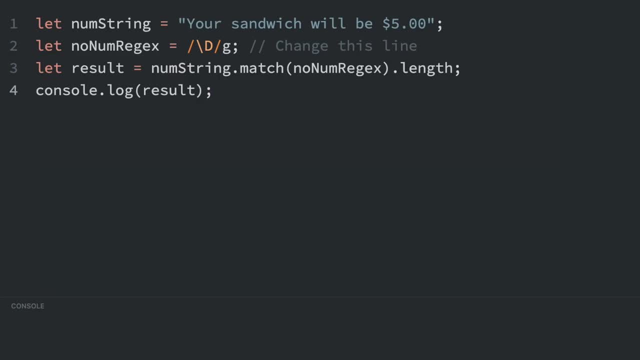 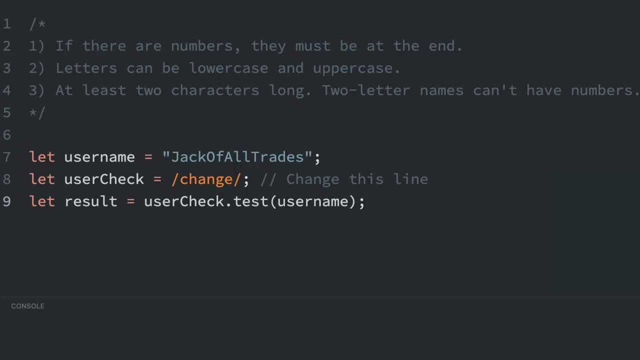 the zero. So we'll run this to get the length of that And we get 24.. We're going to create a regex that can be used as a username validator. In this case, there are three requirements for the username. So here's. 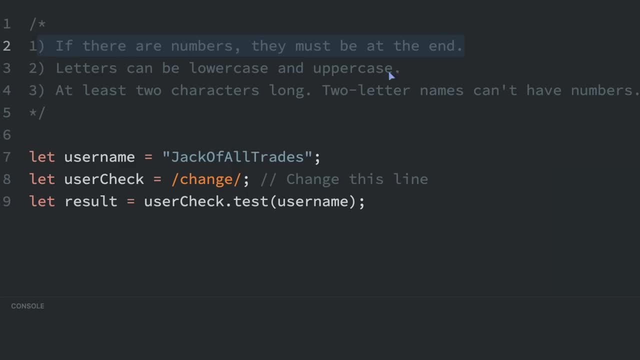 the first requirement: If there are numbers, they must be at the end. Second requirement: letters can be lowercase and uppercase. And then the third requirement is that it must be at least two letters long. two letter names can't have numbers, which is kind of a fourth requirement. So let's 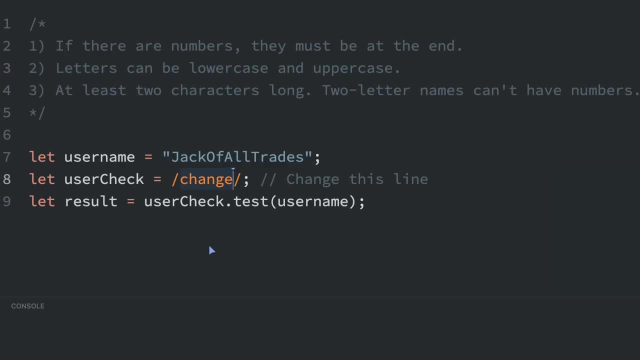 create the regex here. So first we are going to do the requirement that the numbers should be at the end. So if the numbers should be at the end, then letters should be at the beginning. So to specify what's at the beginning, we're going to use the carrot sign And then we're going to 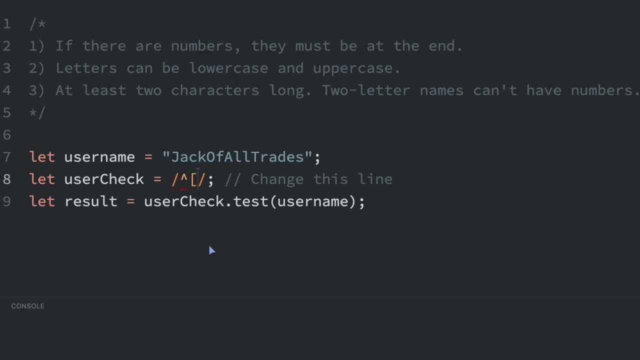 specify the number of letters And then we're going to specify the number of letters at the beginning, which are lowercase and uppercase letters. So I'll do A through Z uppercase and then A, A through Z- lowercase. So now it shows that at the beginning is going to be A through Z. 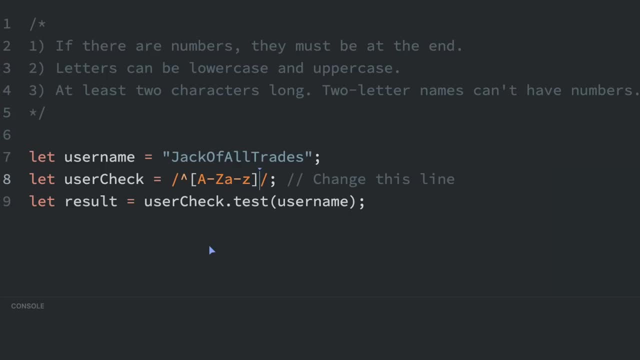 uppercase or A through Z, lowercase, And to specify the number of letters that are going to be at the beginning, we're going to use the following: I'm going to put a curly brace, two comma and curly brace. the curly braces indicate the number of times the previous thing can match. So 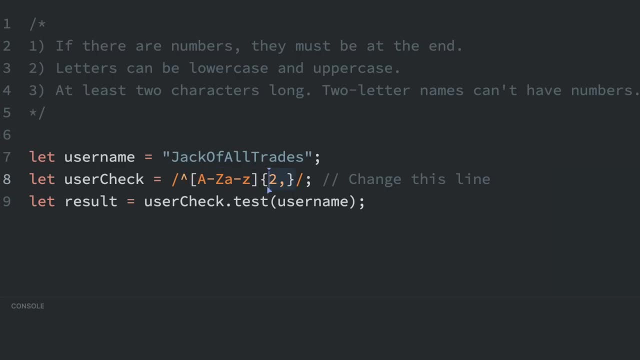 the previous thing are these letters, And these can match anywhere between two and infinite number of times. So the number before the comma is the minimum number of matches And the number after the comma is the maximum number of matches. So we know that every username is going to start with a. 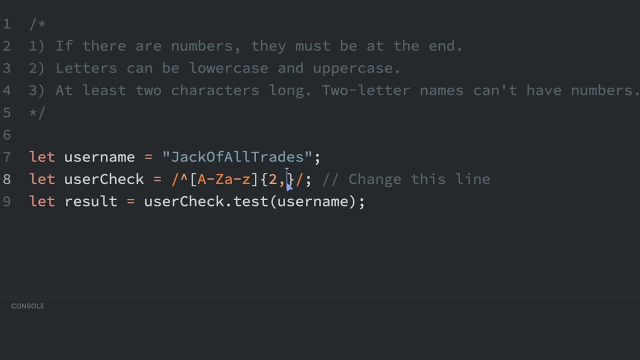 at least two letters, And since there's no number after the comma, it can have an infinite number of letters in the username. If we wanted it to have at max eight letters, then we could put the number eight after the comma, But since we don't care about the max, we're going to leave it as nothing. 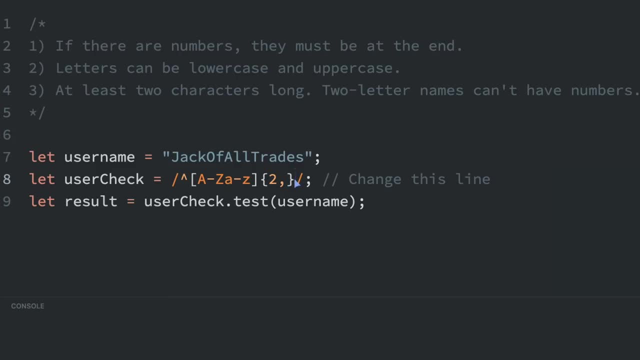 after the comma. So next, we want to show that the numbers must be at the end And you can have any number of numbers. So I'll put slash D, And that represents all numbers. I'll put a star. So this star or asterisk means. 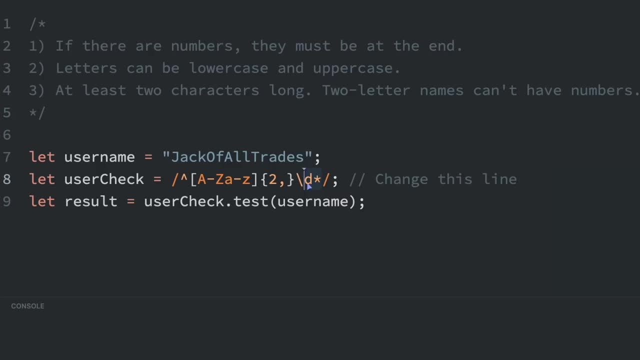 that there should be zero or more. So this means zero or more numbers. And now to show that the zero or more numbers are, at the end I will put a dollar sign. we can now run this regex to make sure a username meets all of these requirements. 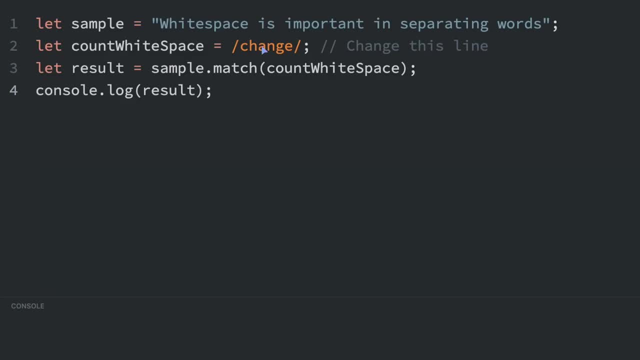 We can match white space characters with slash s. So slash s is going to match a space, a carriage, return, a tab, a form feed and a new line character. So if I add a G for global and run that we will see an array of all the spaces in that sentence. the white space is important in separating words. 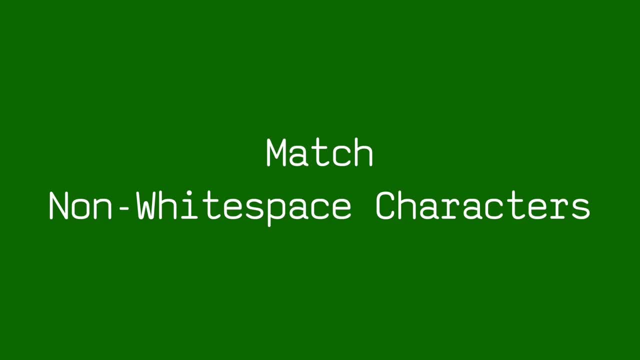 sentence. Now I'll show you how to use the white space. So let's go ahead and run this regex, And now I'll show you how to use the white space. So let's go ahead and run this regex, And now I'll show you how to. 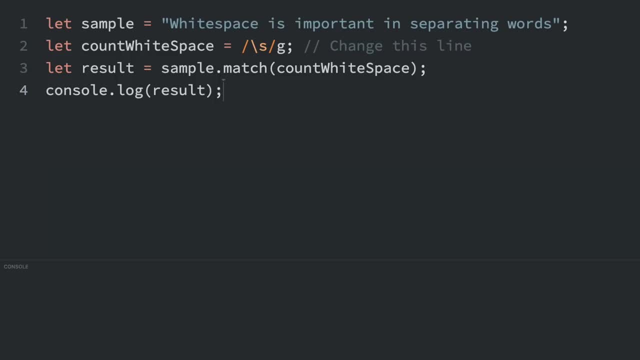 match all non white space characters First make a guess. So remember this is how you match white space characters And if you've been noticing the pattern so far, you'll realize to match non white space characters is just a capital S. So if we run that, you'll see an array of every character. that's. 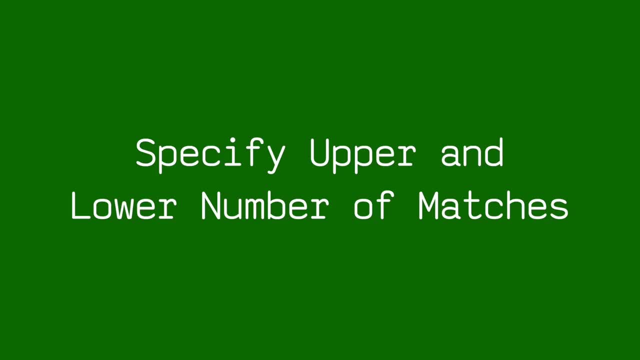 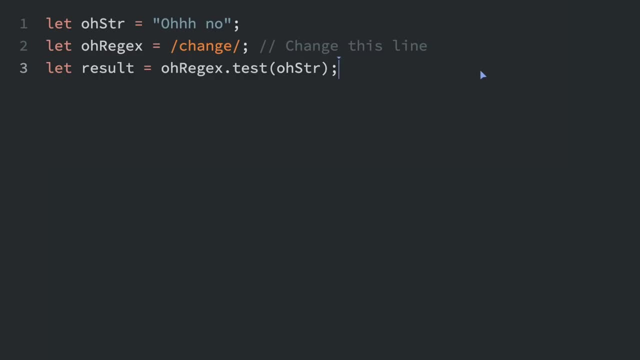 not a space. You can specify the lower and upper and upper number of pattern matches with quantity specifiers. Quantity specifiers are used with curly brackets. I actually talked about these a little bit before. you put two numbers between the curly brackets for the lower and upper number of patterns. So let's say I want to match anything. 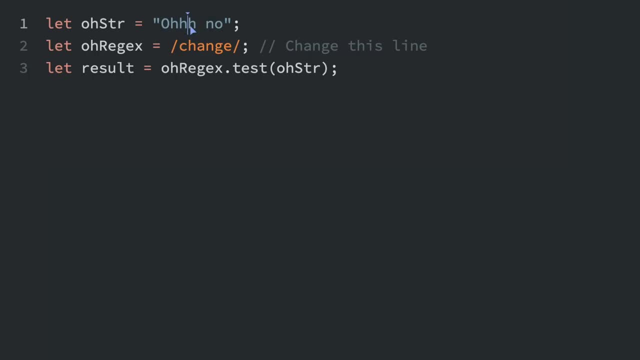 any Oh no, where the number of H's is between three and six H's. So what I'll do is type in the type Oh no, but after the H I'm going to put these curly brackets and put three comma six. So 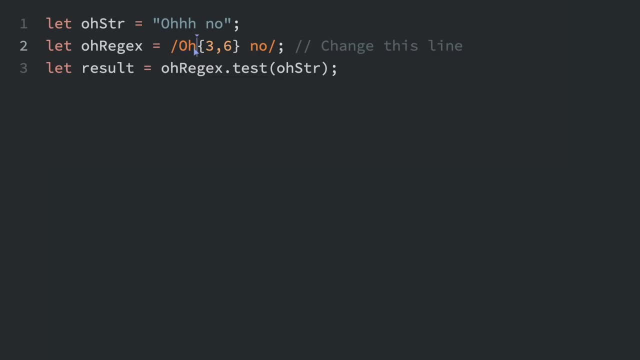 this means we're going to always match the letter O And then we're going to match the letter H, but we only match if there is in between three and six H's, And then we'll also match this space in. Oh, if we had not had a number here and we just had three comma and then nothing in the in curly. 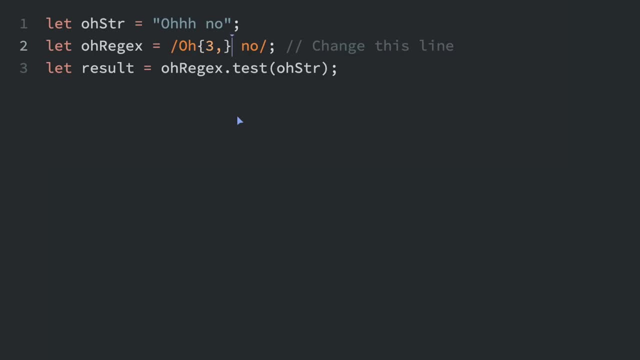 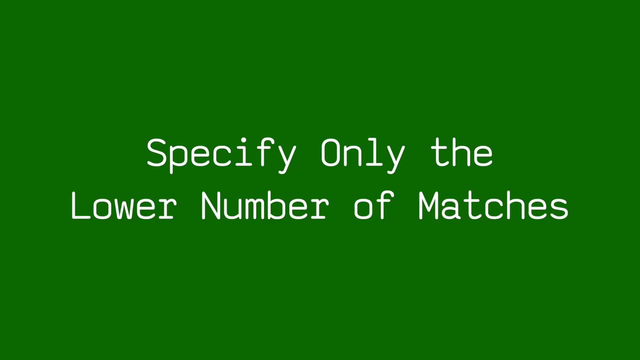 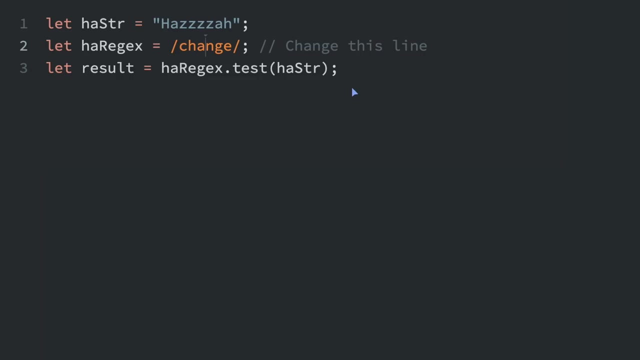 brace, Then it would match for an infinite number of occurrences. So it'd be three H's through an infinite number of H's, But we'll just leave it at six. Here's another example with quantity specifiers where we're going to match four or more of the letter z. So I'll put the letter z. 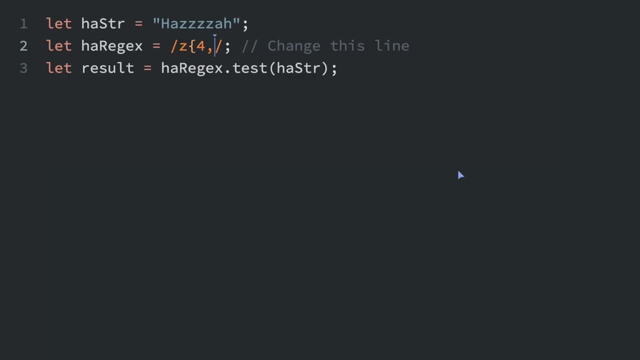 and then the curly brackets. I'll put four comma and then there will be nothing after the comma because, like I said before, when you have nothing after the comma, there's an infinite number that it could go to. So it has to be at least four And then it can be an infinite number of z's. We can use quantity. 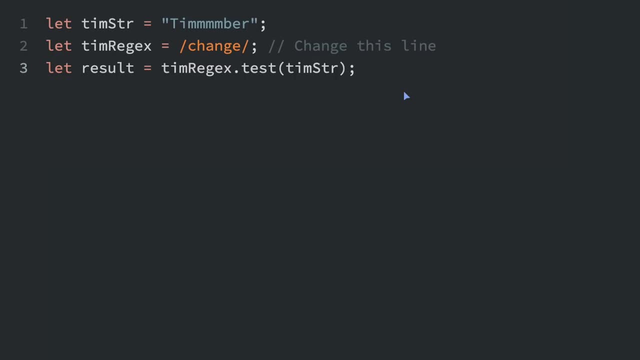 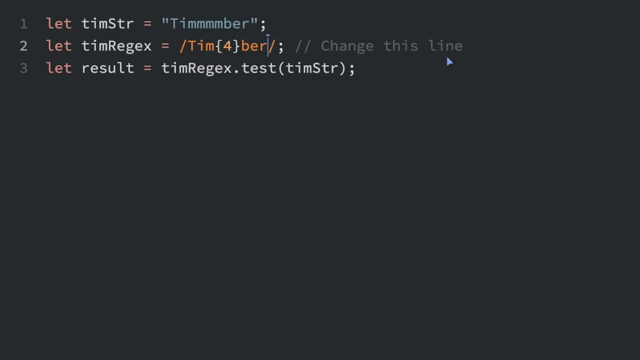 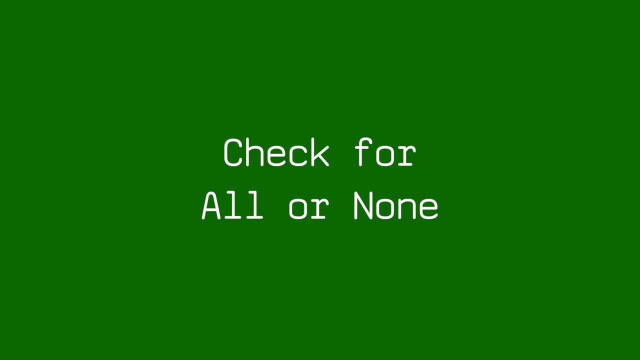 the curly braces and then just put the number four and then ber. So remember before we had the up the lower bound, then comma upper bound. But if we know we want exactly four M's, we can just put the number four in the curly braces. You can specify the possible existence of an. 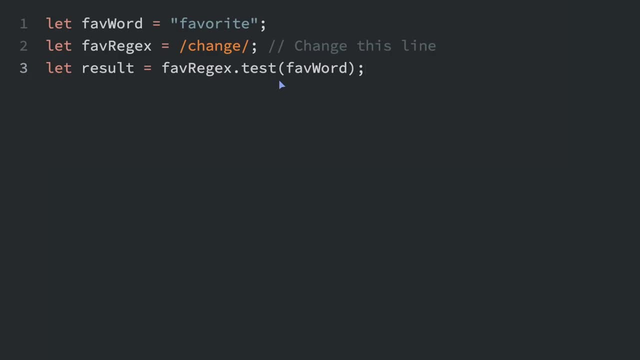 element with a question mark. This checks for zero or one of the preceding elements. It's kind of like saying that the previous element is optional. For example, there are slight differences in American and British English, So the word favorite can be spelled with just an O or with an O, you with British English. So let's create a regex set that searches. 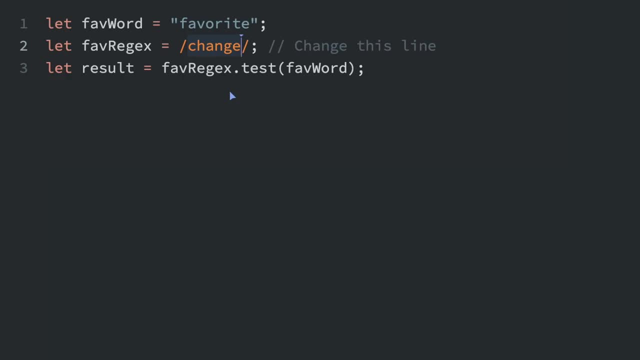 that can match both forms of the word favorite. So do fav, And I'll put a U with a question mark: R I, T, E. So this is this is saying that it may have a U or it may not have a U, but all the other letters have. 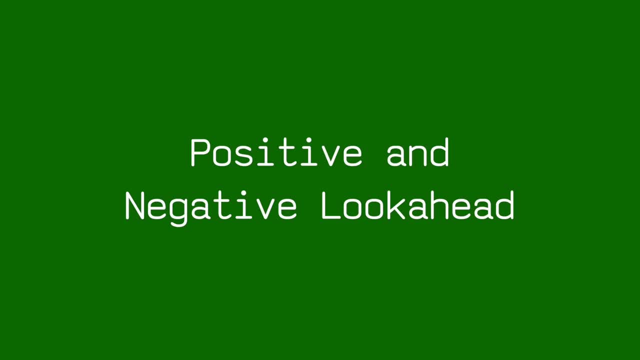 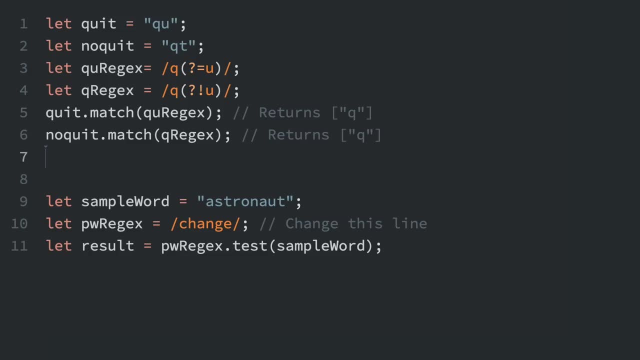 to be the same. Look aheads are patterns that tell JavaScript to look ahead in your string to check for patterns further along. This can be useful when you want to search for multiple patterns over the same string. There are positive look aheads and negative look aheads, So 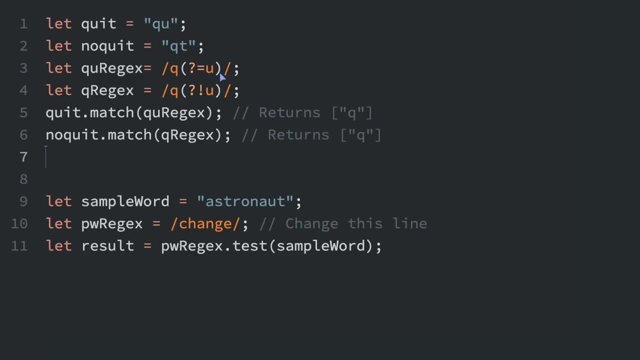 let me show you how they work. So this right here is a positive look ahead. So we have parentheses And then we have a question mark. So the look ahead is always start with a question mark And then it's going to be equals for a positive look ahead or an exclamation point for a negative look. 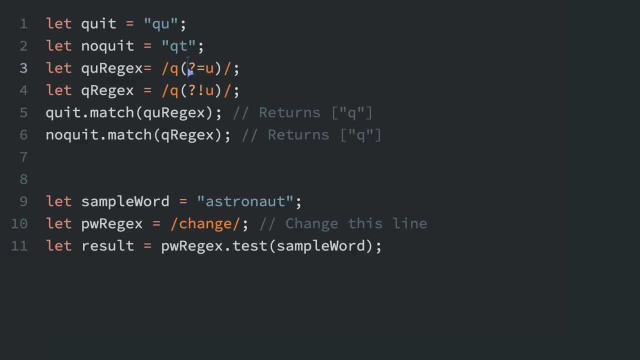 ahead. So let's look back at the positive look ahead. So question mark equals means a passive Look ahead and you have parameters. Let's say: respect. This is the arrow, Derrick, and I'll put a example on your screen. Let's define a positive look ahead. You can change it as so and Ica weak. 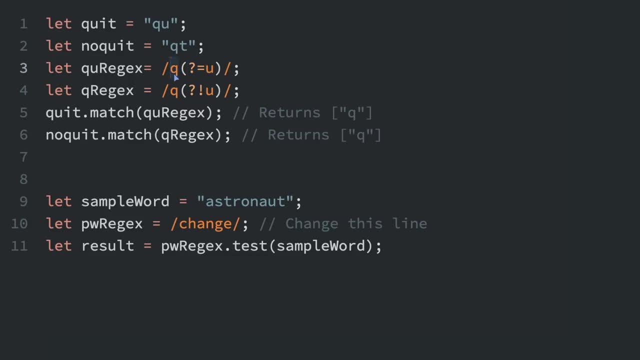 which is an exclamation point. The word closet means a positive look ahead. The word closet is an Cho % change. So it's first going to check for the Q And it's going to look ahead to make sure there is a U later in the string, And if there is a U later in the string, we'll return just the Q. So when we 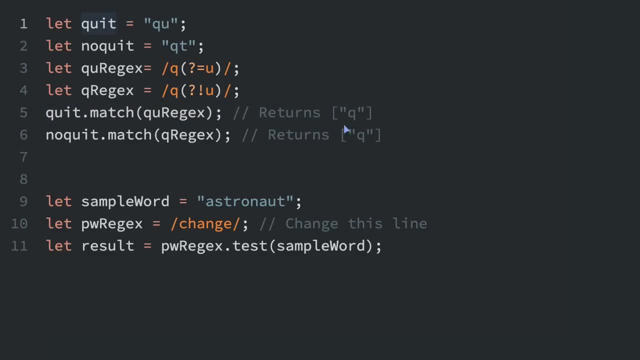 run this regex on the quit string. it's going to return Q because it finds the U later in the string. but it doesn't return that. you a negative look ahead. it's going to make sure that something is not later in the string. So here it's going to search for a Q and make sure there's not a U. 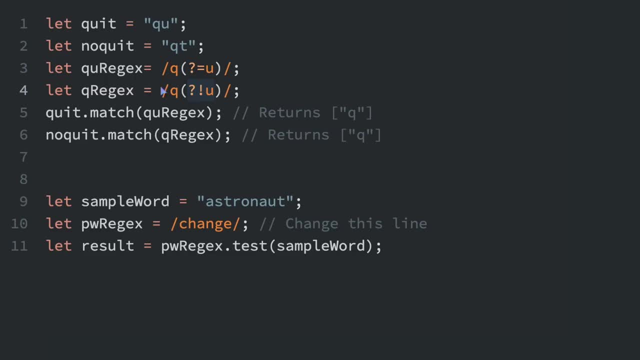 later in the string And if there is not a U later in the string, it's going to return this. So when we run this, look ahead on the no quit screen string. it's going to find the Q and it's going to look ahead and find out there is no U. 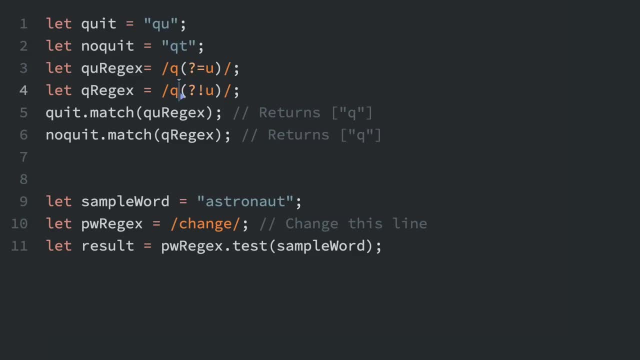 Since there is no U, it's just going to return the queue, because that's what we have before the parentheses. And it's going to return the queue here. a more practical use of lookaheads is to check two or more patterns in one string. So down here, in this example, we are going to use the. 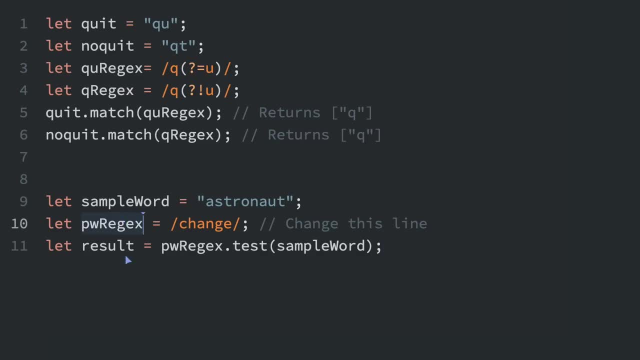 lookaheads in the PW regex to match passwords that are greater than five characters long and have two consecutive digits. So for a greater than five characters we'll do parentheses And then it's always going to start with the question mark equals if it's a positive look ahead, and I want greater than five characters. 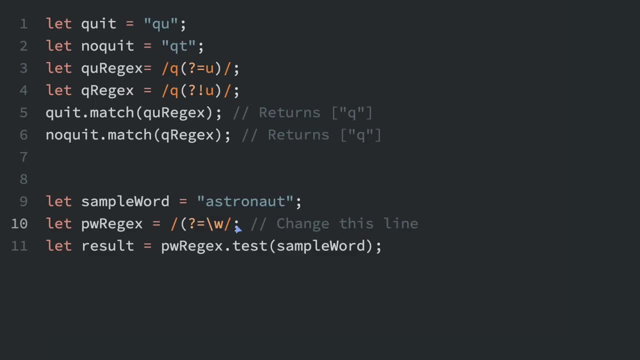 So slash w would be all numbers and letter characters, And we want there to be five characters, at least five characters, And then we also want two consecutive digits. So I'm going to make a another look ahead: question mark equals and we're going to say there can be any number of characters. 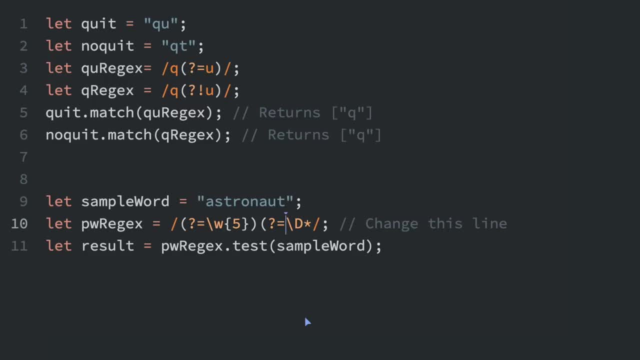 that are not digits. this capital D, the slash capital D, is a character that's not a digits And the asterisk means there's zero or more characters that are not a digit. But we also want to make sure that there are two or more digits, So we have the slash D to 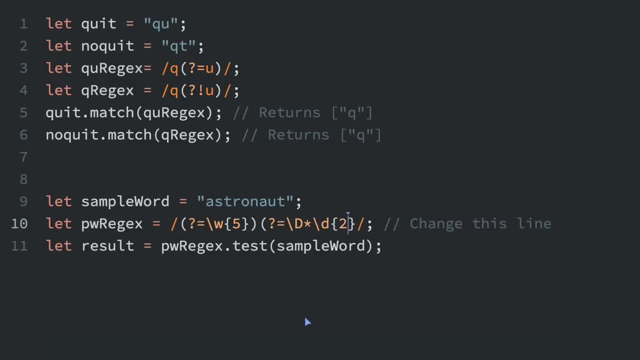 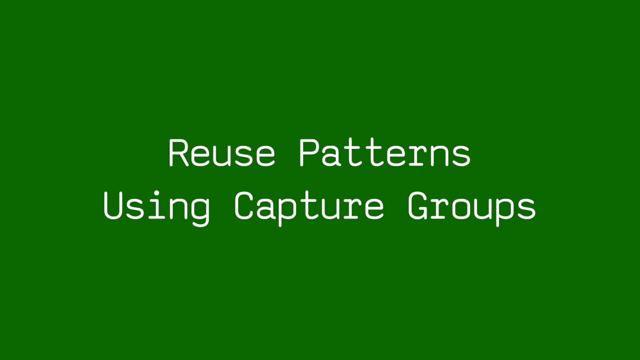 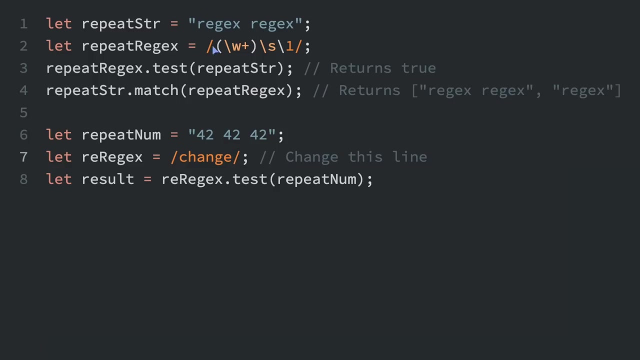 say that there are going to be digits and then we have two, so there's gonna be two or more digits. So this is going to match for five or more characters and then two or more digits. You can group things you are searching for in a regex with parentheses. So here we have parentheses around here, So we are. 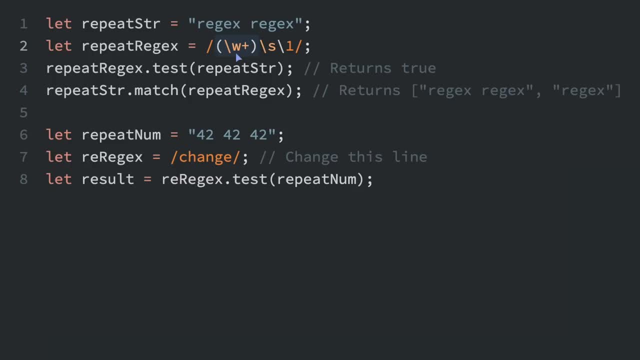 searching for any number of characters And then after that there's going to be a space. You can also use these parentheses to repeat substrings. So this is called a capture group And you can repeat this group any number of times. So in this regex we have this first group in parentheses and we can repeat that first. 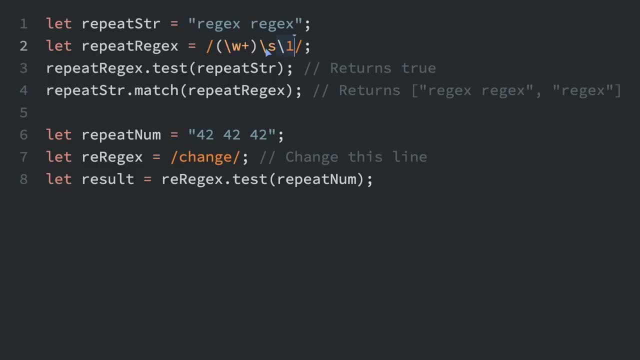 group with a slash one. If we had a another group with parentheses, we can repeat that second group with slash to. So in this case we are searching for any group of any number of letters followed by a space, followed by any number of letters that are the. 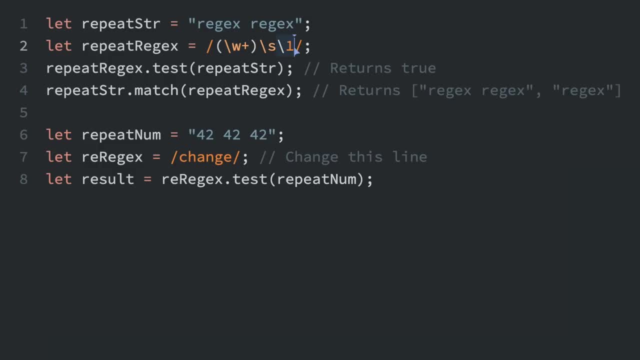 same letters as before, because we're doing slash one. If we test this regex against this string, it's going to true because it has any number of letters, it has a space, and then it repeats any number of letters, the same letters from before. So that's any number of letters, the space, and then we're repeating. 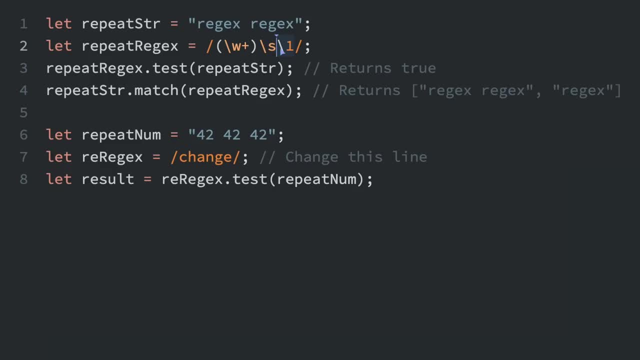 the same letters as before. Now here, where we did slash one, we could have just put this whole thing again. the parentheses with the slash W I'm going to copy and paste here. So this would have been the same thing. But instead of repeating this twice, we can just put slash one to save. 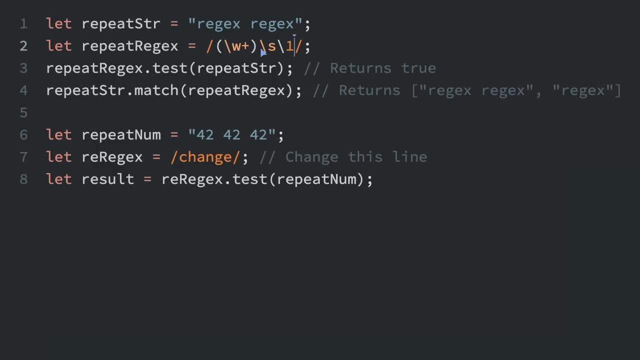 space. So we don't have to repeat, if we want to repeat, the same search over and over again in a in a regex. So if we look down here for the match, at first this may seem confusing what it's returning. But what it's returning, the first element in the array is the full match. 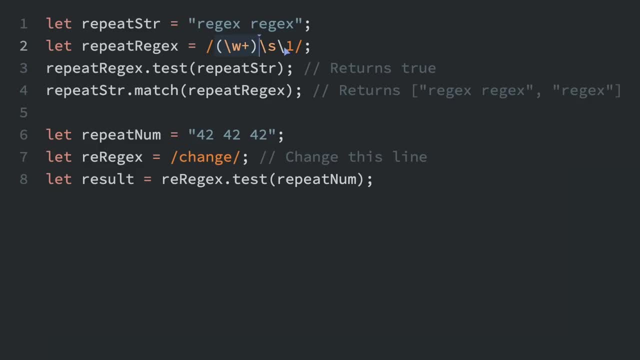 So that's the, the any number of characters plus a space, plus any number of the same characters. So the full match is this. And then the second element in the array is just whatever is in the capture group- This is the capture group And we- and what's in the capture group is just regex. 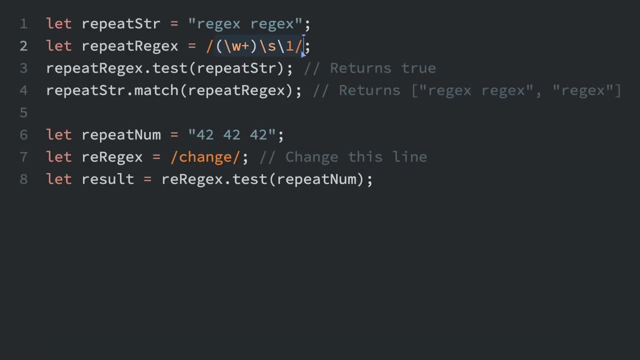 That's why we have regex- regex, which is the full regex, And then the second element of the array is just regex, which is just the capture group, the thing in the parentheses here. So down here we are going to attempt to use capture groups to match numbers. 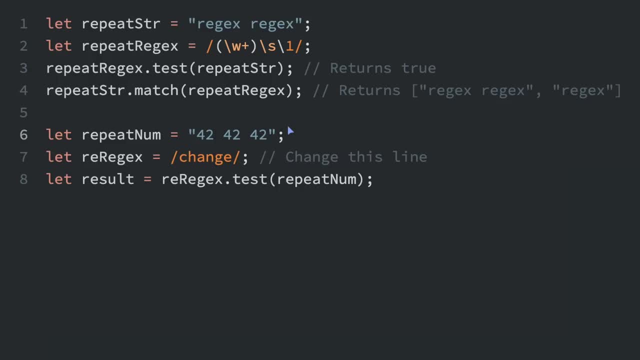 that are repeated only three times in a string each separated by a space. We want this regex to match something like this: 42 space, 42, space, 42.. We would also want it to match something like: 136 space, 136, space, 136.. It doesn't matter what the number is, And we only want to match a group. 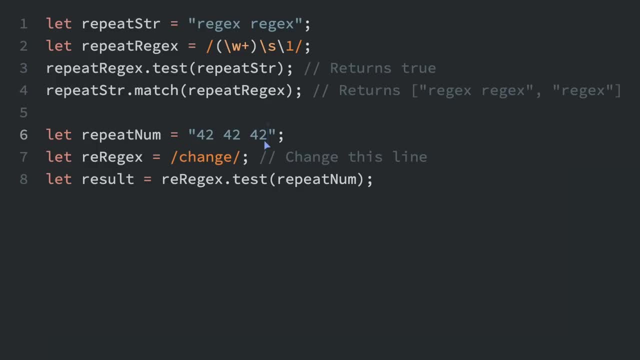 of three. So we don't want to match a group of three. So we don't want to match a group of three. We want to match four numbers, five numbers, six numbers, just a group of three numbers separated by spaces. So let's see how to do that. We are going to use a capture group, So I'm going to 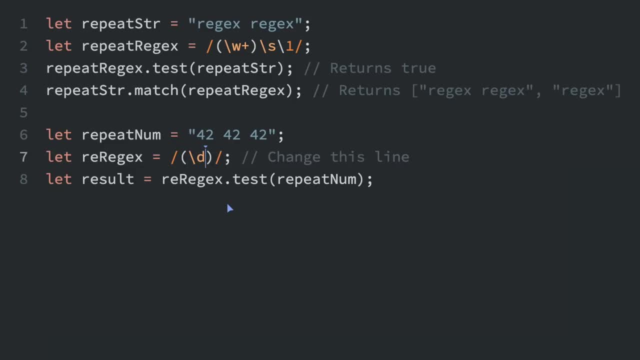 put a parentheses, slash. D plus that means any number of digits, And that's going to be the end of our capture group, And then it's going to have a space, And then I'm going to put slash one, which just is a shorthand way of repeating the first thing. 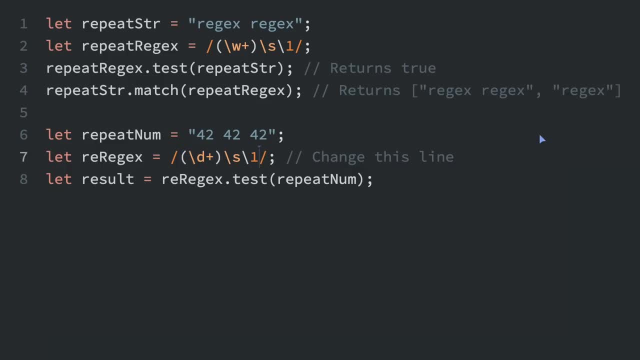 in parentheses, which is this: And then we'll have another space and another slash one. So this is going to look for any number and a space, any number, and a space, any number, So it's a number three times. We're not quite done yet, though, Because, remember I say, said we want to match. 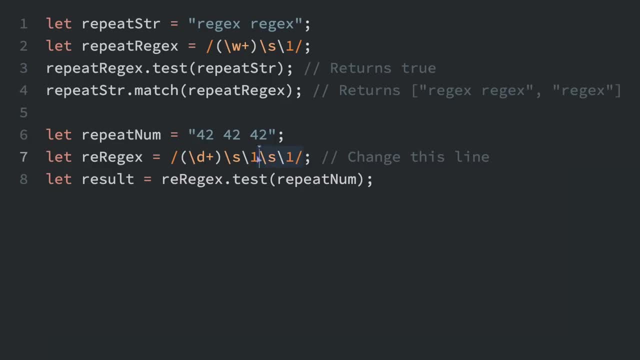 only three numbers. So this regex would also match this if the number was in there four times, because it would find 4242, 42. And then stop, and it would say, Oh, we found it, But we don't want to match it. If there's four 42s in a row, we only 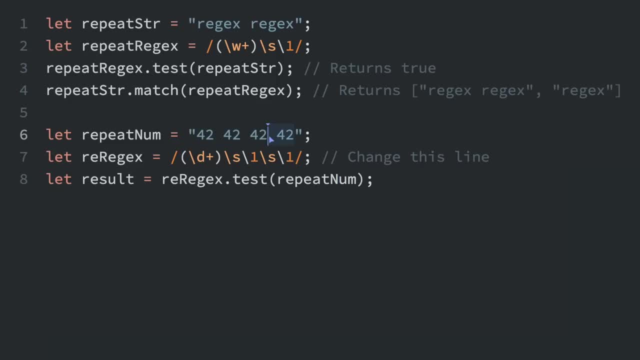 want to match it. we only want this to return truth. there's three 42s in a row, So that's simple to fix. We just have to have a bracket, or I mean a carrot at the beginning and a dollar sign at the end. So remember, a carrot means that we want this at the beginning of the string And then 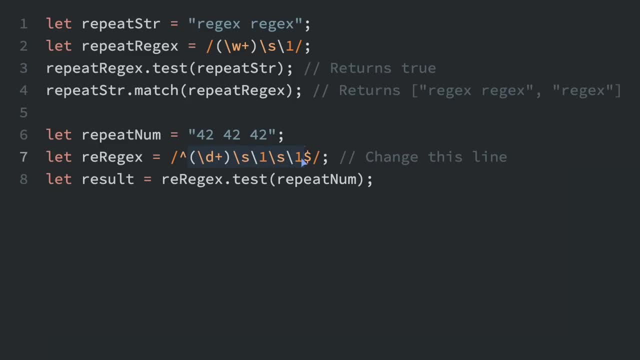 a dollar sign means we want this at the end of the string. So adding the care and the dollar sign just means we want exactly this. we don't want anything before this. we don't want anything after this. So now this will return. true for any group of three numbers, not a group of four numbers, not. 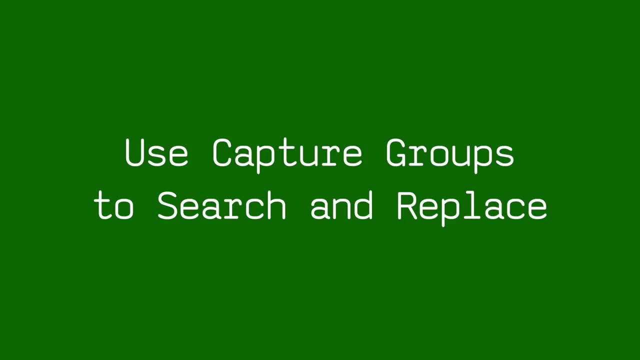 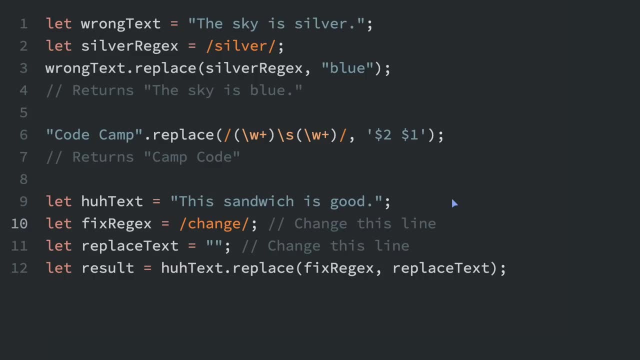 a group of five numbers. You can search and replace text in a string using the replace function on a string. The inputs for replace is first the regex pattern you want to search for And the second parameter is the string to replace, the match or a function to do something. So let's look at this example. we have this text: 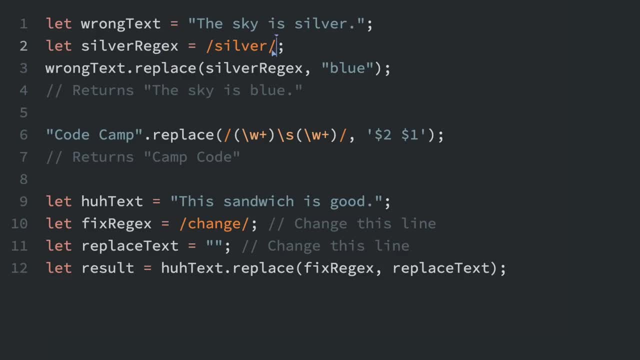 the sky is silver. we're going to search for silver. this is our regex pattern, So we're going to do a replace. And then we're going to search for silver. And then we're going to do a replace. Here we've got the wrong text: dot replace. we're going to pass in the regex the silver regex. 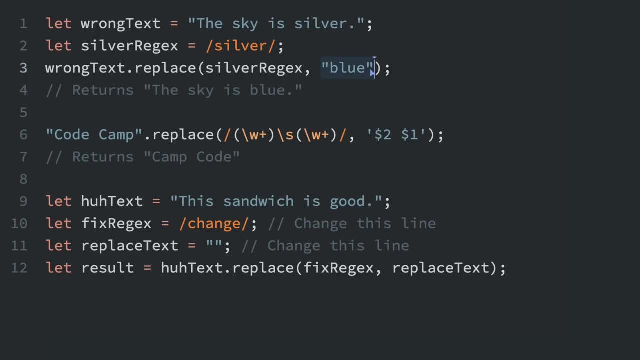 which is searching for the word silver, and it's going to replace it with the word blue. So this is going to return. the sky is blue. Now you can also access capture groups in the replacement string with dollar signs. Let me show you what I mean down here. So here we have a string code. 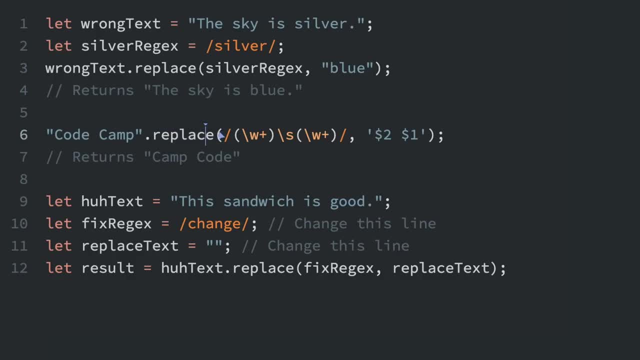 camp, And then we're going to call the replace function on that string, And then we're going to call the replace function on that string. Now look at the regex. So up here we just use the variable silver regex which was set to this regex. Here we're putting them in the regex. 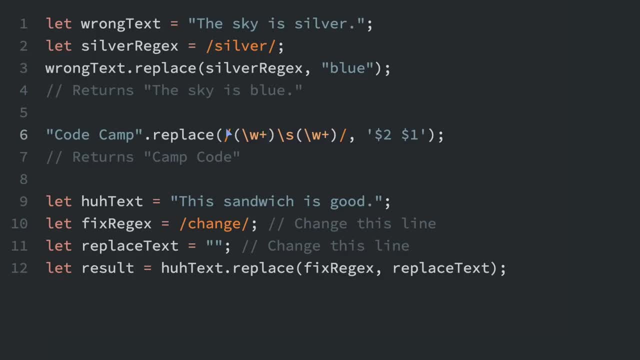 directly into the function instead of using a variable. So look at this regex. we have this capture group, which just means any number of letters, then we have a space, And then we have this other capture group, which just means any number of letters. So that's going to find this. 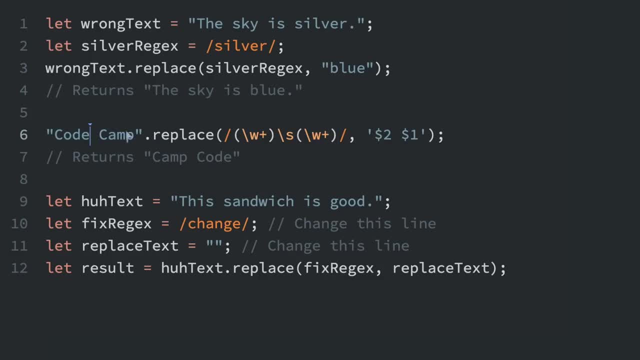 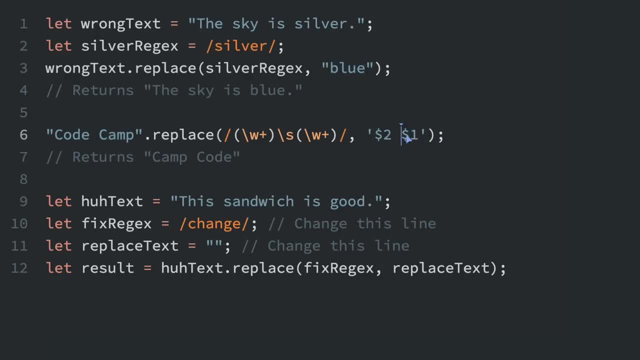 we just put in the word we want to replace with. But here we do something different. It says dollar two, dollar sign one. So dollar sign two means the second capture group, the second parentheses in the regex. So the second capture group is this, which has matched to the word camp. 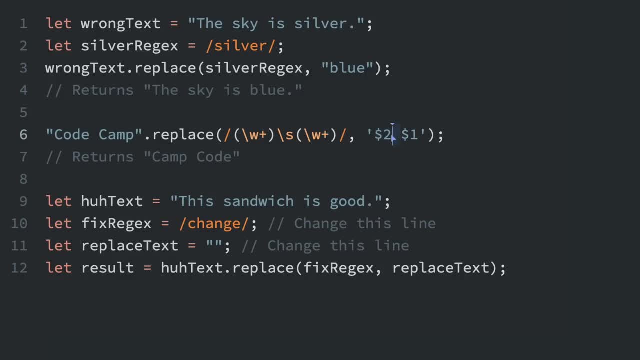 So we're putting camp at the beginning and then a space And then dollar sign. one means the first capture group, which is this section which matched the word code. So this is a way, so you can see it returns camp code. So we pass in the text code, camp, and it returns camp code. So that's. 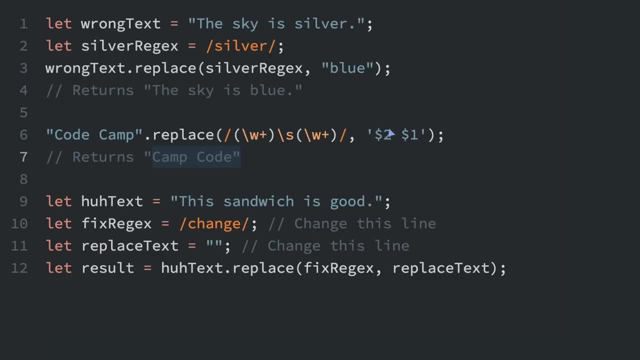 another cool thing you can do with capture groups when you're doing a replace. So let's get back to the easier one up here. we're going to actually make some changes down here. that follows this pattern up here. So this sandwich is good. Well, we are going to find the word good here And we're 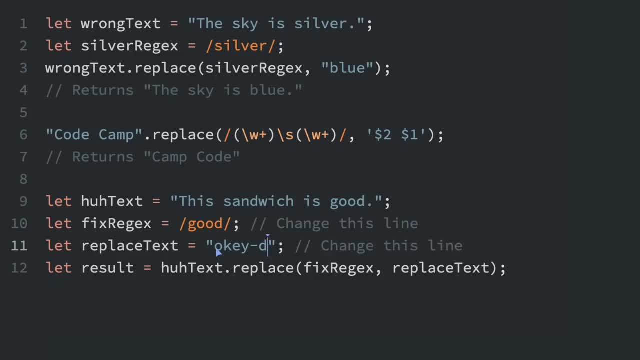 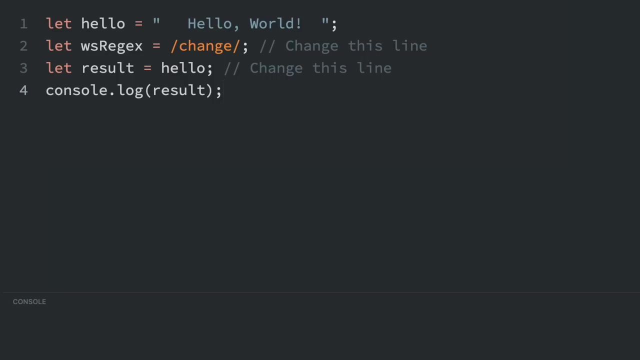 going to replace it with the word okie dokie. So here it's going to find the fixed regex, which is good, And it's going to replace it with the replace text, which is okie dokie. This is a regex coding challenge. The challenge is to write a regex and use the appropriate string. 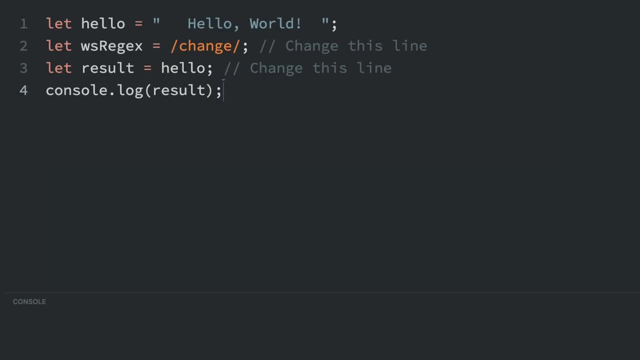 methods to remove white space at the beginning and end of this string here. Now, the trim method would work here, But the challenge is to do it with just using regular expressions. So we are going to do a replace. But we have to write a regular expression, So we're going to do a replace. 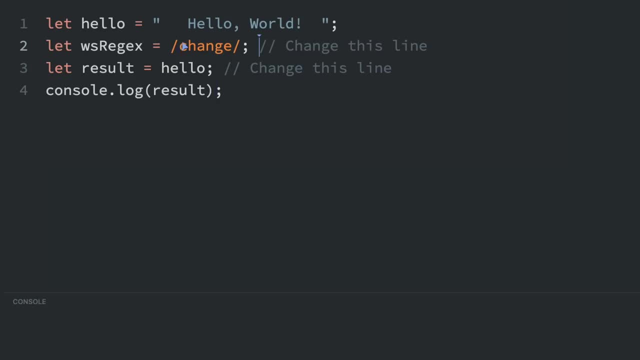 That's going to figure out what we're going to replace. Well, let's write a regular expression that finds all the space at the beginning and all the space at the end. So this is how we'll do this: To find everything at the beginning. it's going to start with a carrot which finds